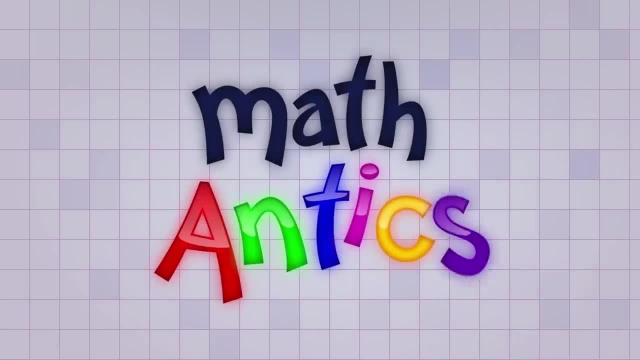 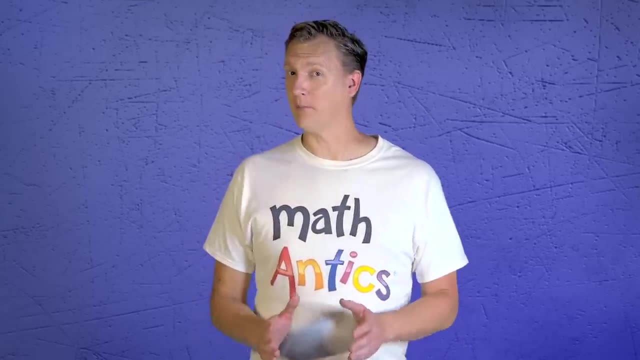 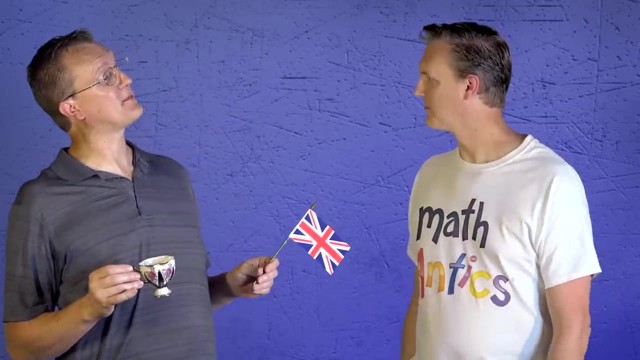 Hi, welcome to Math Antics. In this lesson we're going to learn about an important math concept called exponents. Sounds kind of weird, huh? Indeed, it does, my good man, And I'm afraid it's because you're pronouncing exponents incorrectly. 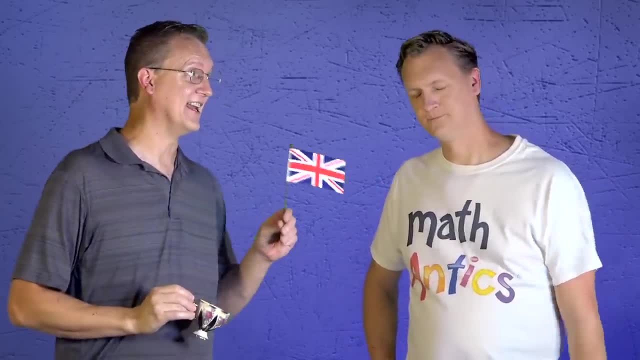 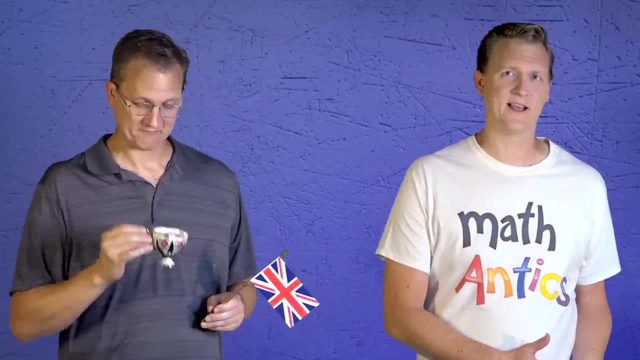 The proper pronunciation is IN-DE-CEES. IN-DE-CEES- Oh yeah, that's right. In a lot of countries, exponents are called IN-DE-CEES, But the good news is that the concept is the same, no matter what term is used. 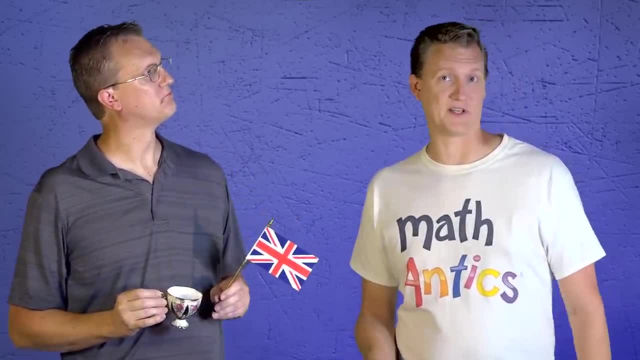 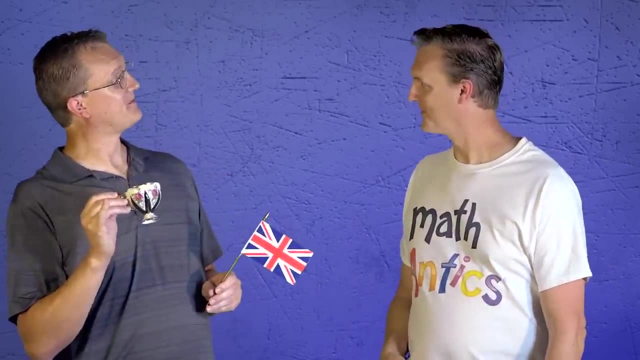 And since I'm usually an American, I'll usually use the term exponents in this video, But I'll occasionally point out the other terminology too. Sound good to you? Jolly good, sir, Toodle-pip. Alright then, but what are exponents or IN-DE-CEES? 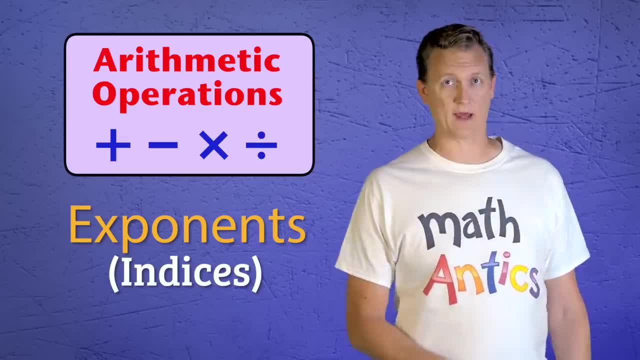 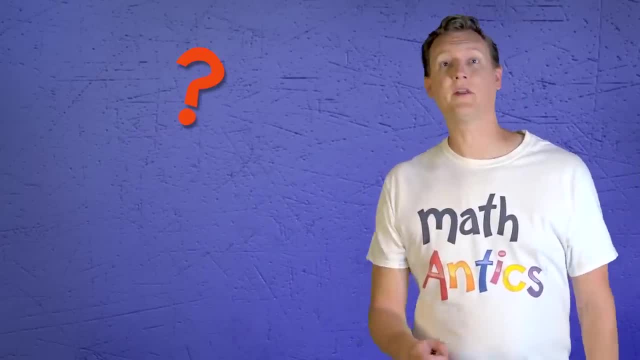 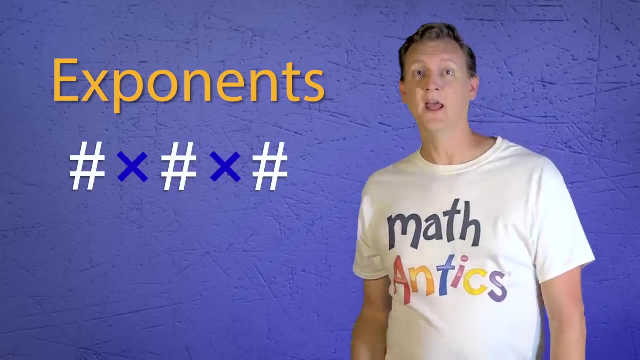 Well, just like the four main arithmetic operations that we use in math, exponents are a type of math operation. They tell us what to do and what not to do. OK, but what do they tell us to do? Exponents tell us to take a number and multiply it by itself a certain number of times. 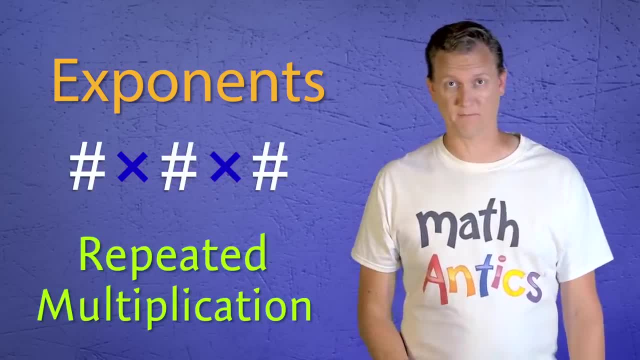 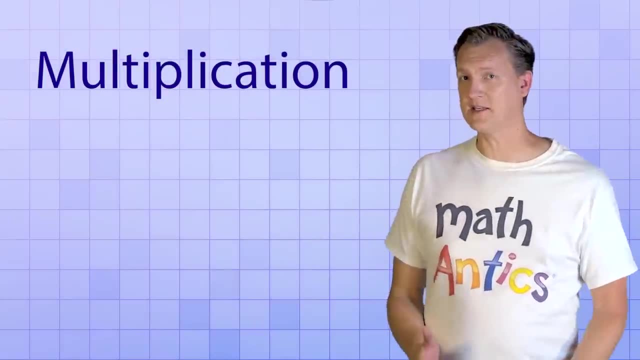 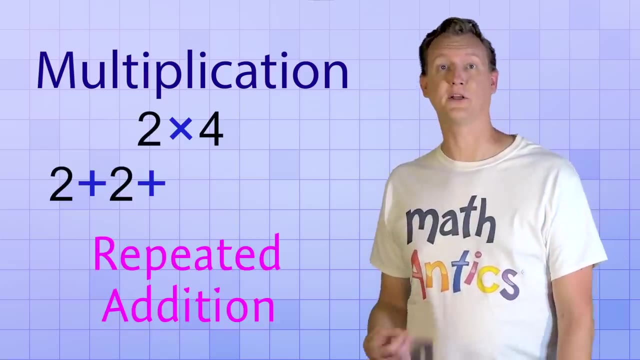 In other words, exponents are basically repeated multiplication. To help you understand what I mean, let's review multiplication for just a second. Do you remember how multiplication is basically repeated? addition, For example, 2 times 4, is the shorthand way of writing 2 plus 2 plus 2 plus 2.. 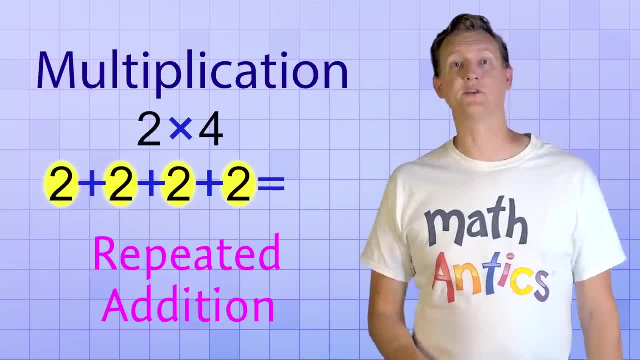 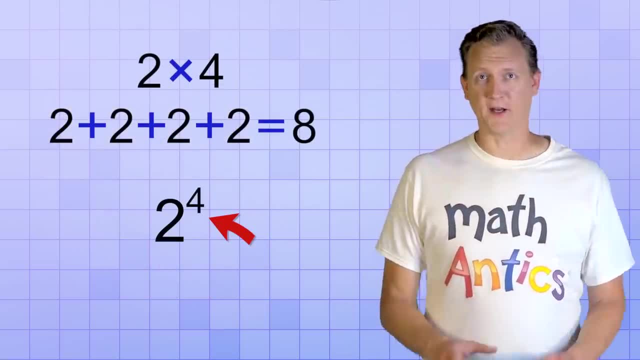 It's the same as 4 2's being added together, which equals a total of 8.. Now let's compare that to a similar exponent: Yep. that's an exponent, and in a minute we'll talk about why it looks like that and why the numbers are different sizes. 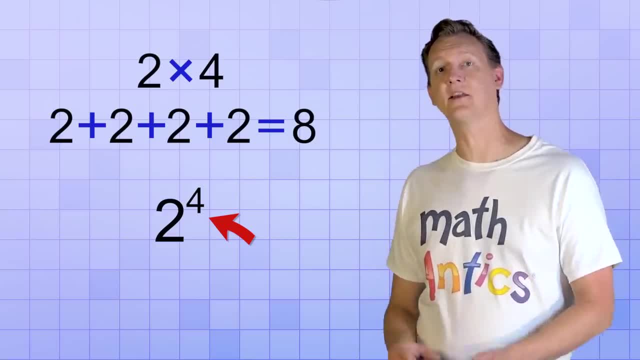 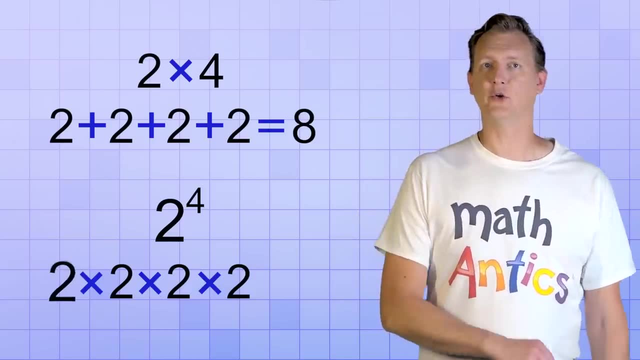 But for now, you just need to know that this exponent tells us to take the number 2 and multiply it 4 times. In other words, you would take 4 2's and multiply them together 2 times 2 times 2 times 2,, which would equal 16.. 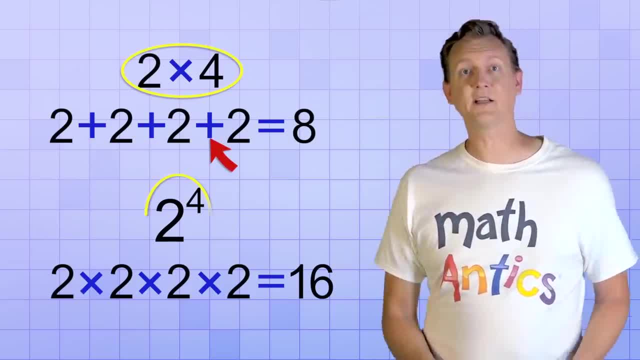 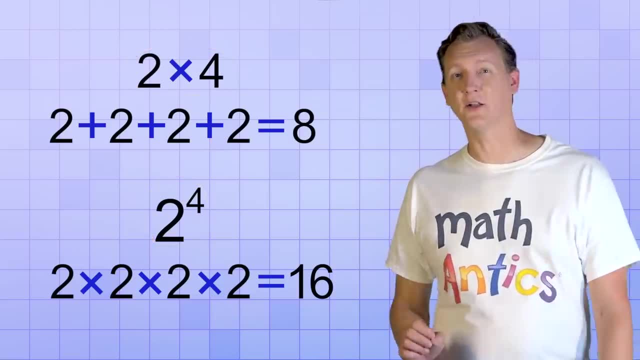 So multiplication shows repeated addition and exponents show repeated multiplication. And we'll see more examples of how exponents work in a minute. But first let's talk a little bit about why exponents look the way they do. Exponents involve two numbers. 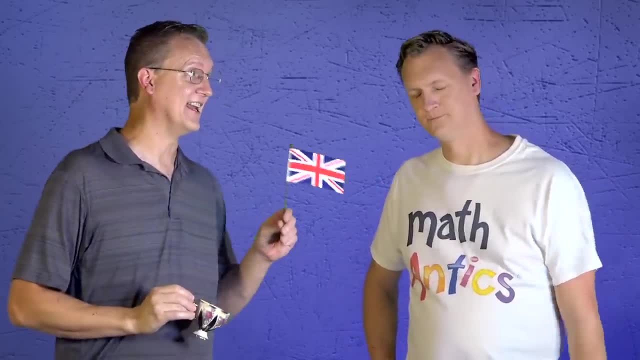 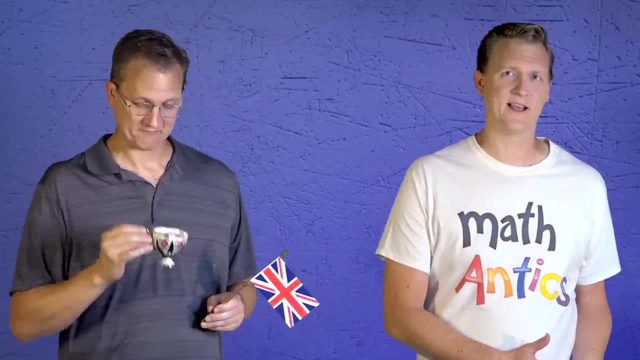 The proper pronunciation is IN-DE-CEES. IN-DE-CEES- Oh yeah, that's right. In a lot of countries, exponents are called IN-DE-CEES, But the good news is that the concept is the same, no matter what term is used. 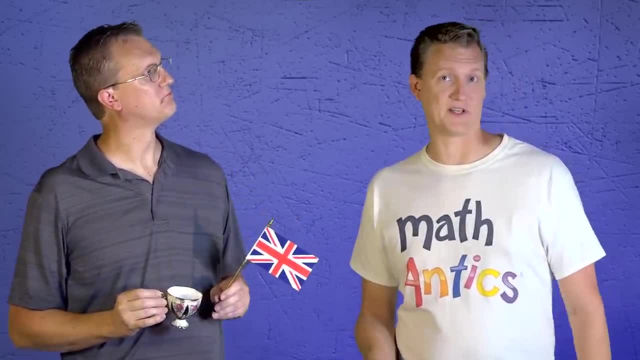 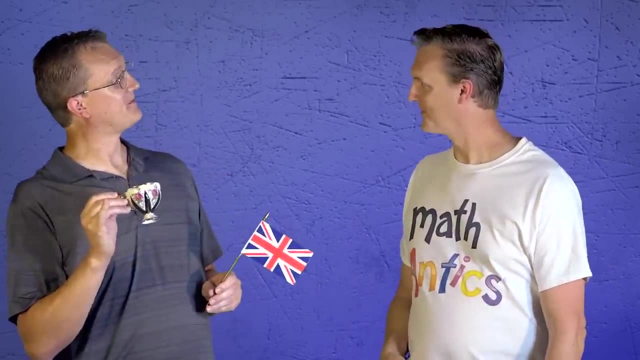 And since I'm usually an American, I'll usually use the term exponents in this video, But I'll occasionally point out the other terminology too. Sound good to you? Jolly good, sir, Toodle-pip. Alright then, but what are exponents or IN-DE-CEES? 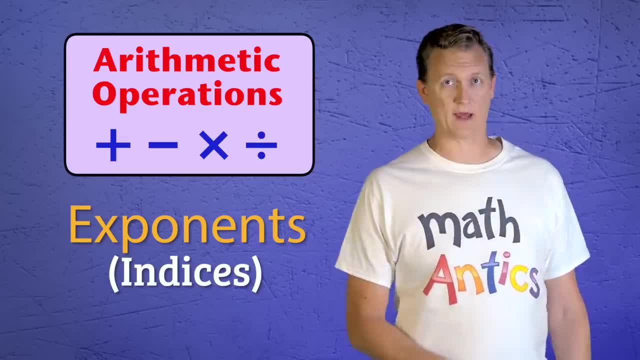 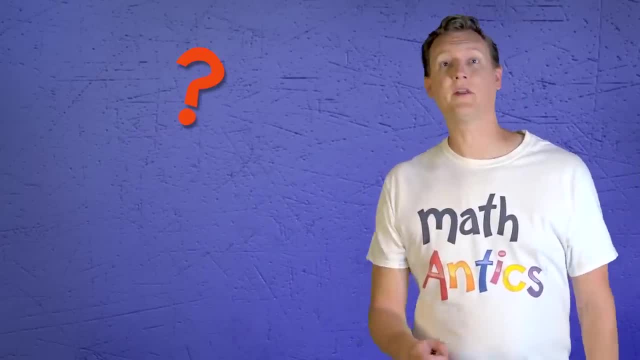 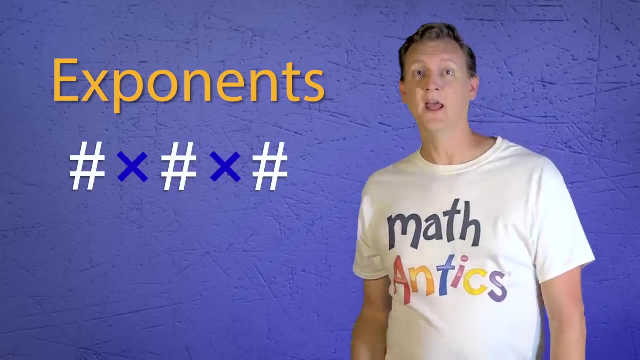 Well, just like the four main arithmetic operations that we use in math, exponents are a type of math operation. They tell us what to do and what not to do. OK, but what do they tell us to do? Exponents tell us to take a number and multiply it by itself a certain number of times. 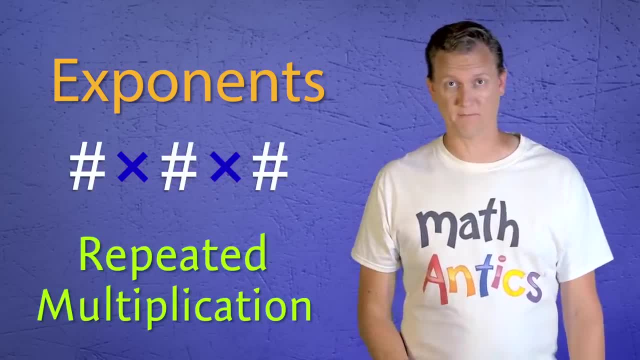 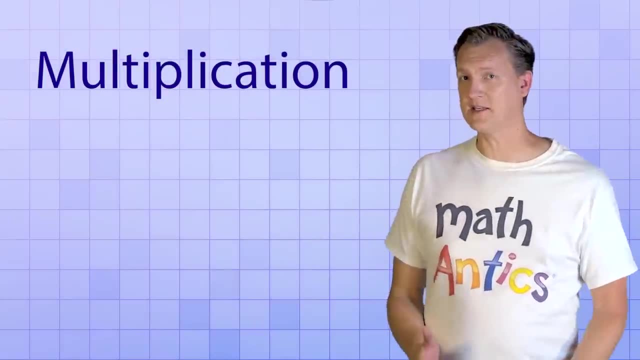 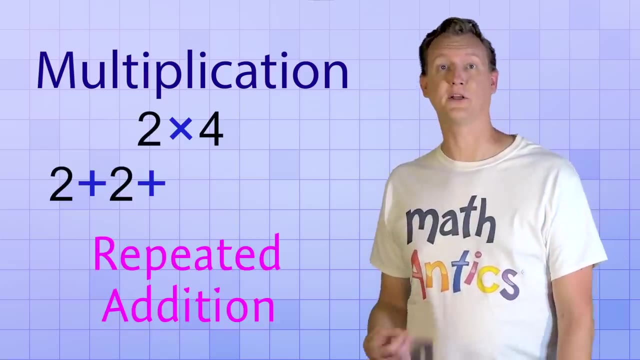 In other words, exponents are basically repeated multiplication. To help you understand what I mean, let's review multiplication for just a second. Do you remember how multiplication is basically repeated? addition, For example, 2 times 4, is the shorthand way of writing 2 plus 2 plus 2 plus 2.. 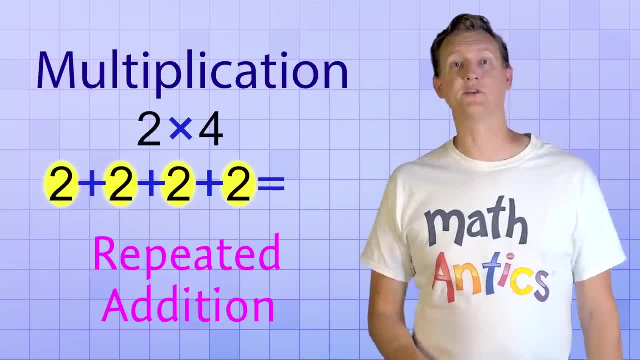 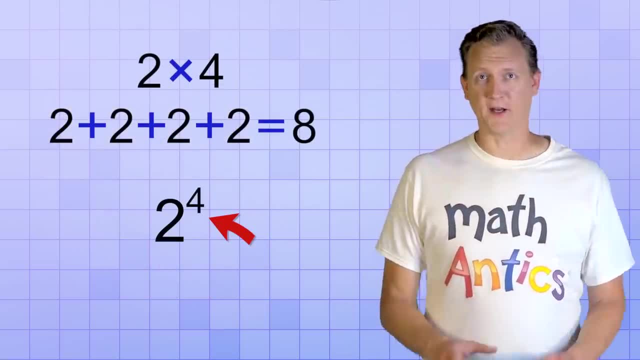 It's the same as 4 2's being added together, which equals a total of 8.. Now let's compare that to a similar exponent: Yep. that's an exponent, and in a minute we'll talk about why it looks like that and why the numbers are different sizes. 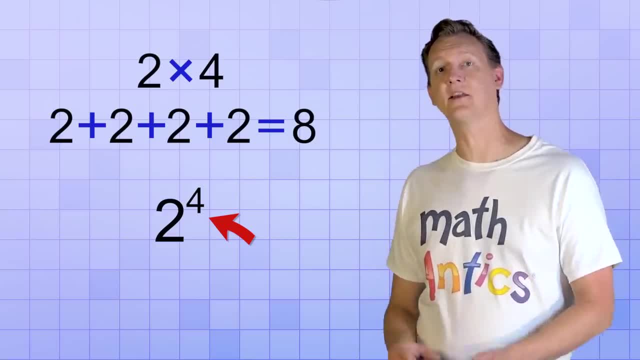 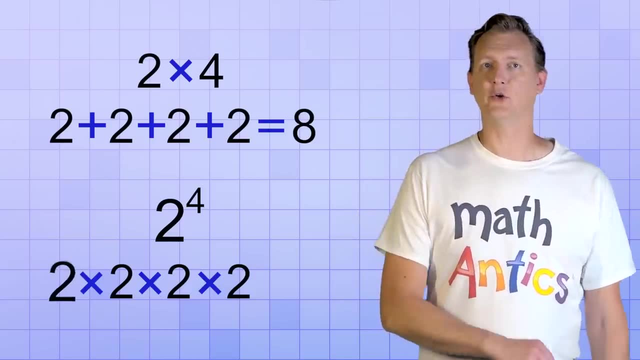 But for now, you just need to know that this exponent tells us to take the number 2 and multiply it 4 times. In other words, you would take 4 2's and multiply them together 2 times 2 times 2 times 2,, which would equal 16.. 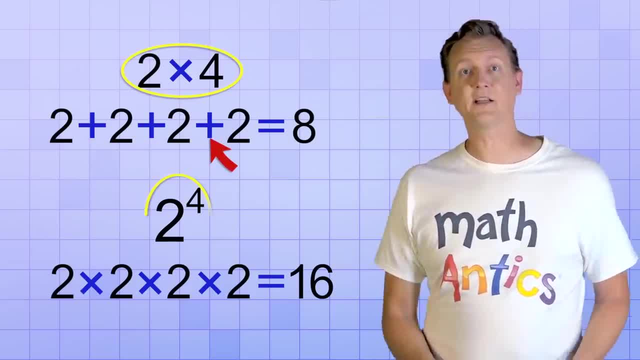 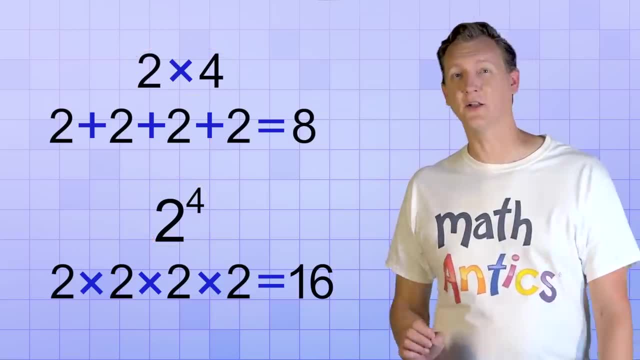 So multiplication shows repeated addition and exponents show repeated multiplication. And we'll see more examples of how exponents work in a minute. But first let's talk a little bit about why exponents look the way they do. Exponents involve two numbers. 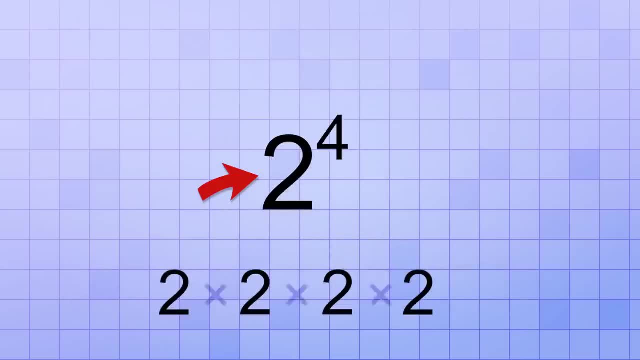 The first number is the one that gets multiplied repeatedly a certain number of times and it's written full size and it's called the base. The second number tells us how many copies of the base to multiply together. It's written much smaller and up at the top of the line like this: 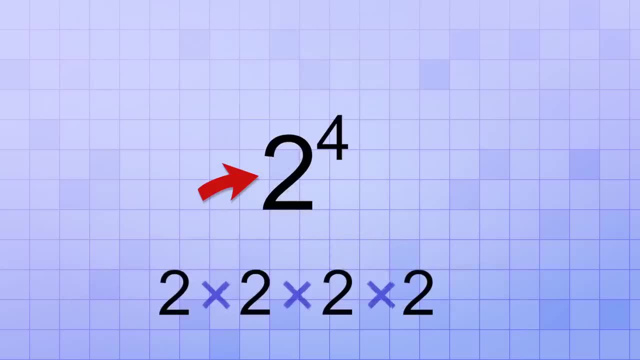 The first number is the one that gets multiplied repeatedly a certain number of times and it's written full size and it's called the base. The second number tells us how many copies of the base to multiply together. It's written much smaller and up at the top of the line like this: 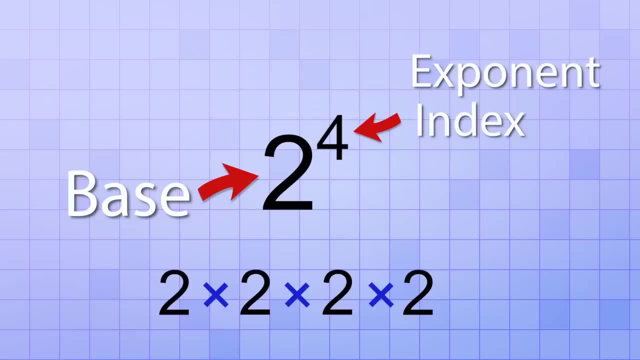 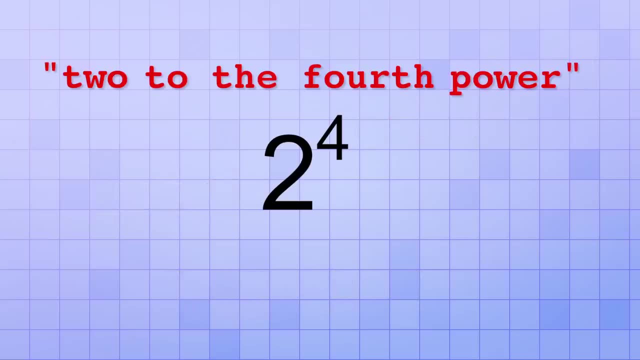 And it's called the exponent or the index, And when reading exponents some interesting terminology is used. This exponent would usually be read 2 to the 4th power, or just 2 to the 4th, for short. And this exponent would be read 3 to the 5th power, or just 3 to the 5th. 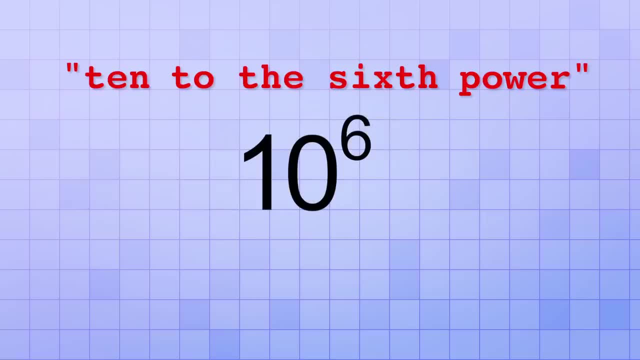 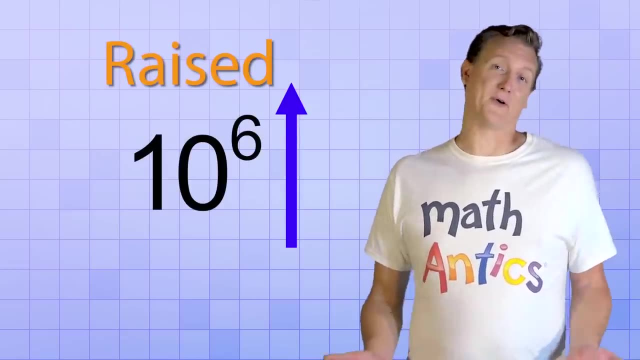 And this exponent would be read: 10 to the 6th power, or just 10 to the 6th, Get the idea? Oh, and you'll often hear people say that a number is raised to a certain power, You know cause. it sounds kinda cool. 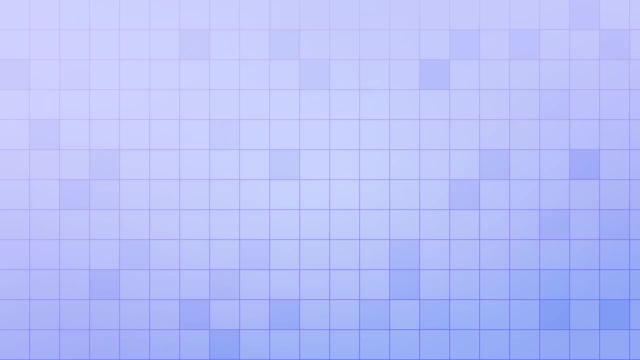 But it's just another way of saying the same thing. Unfortunately, that terminology has created a little confusion. Traditionally you'd say you have a base raised to a number, called an exponent, and the answer you get by doing that is called a power of that base. 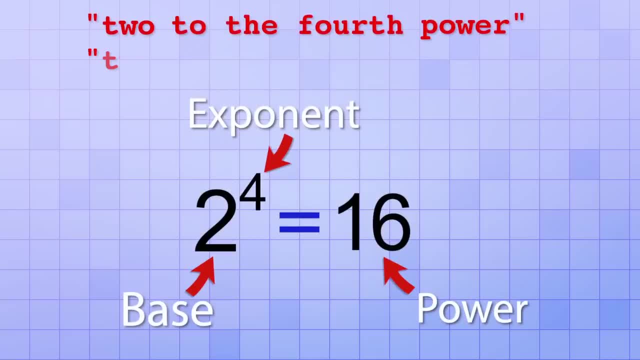 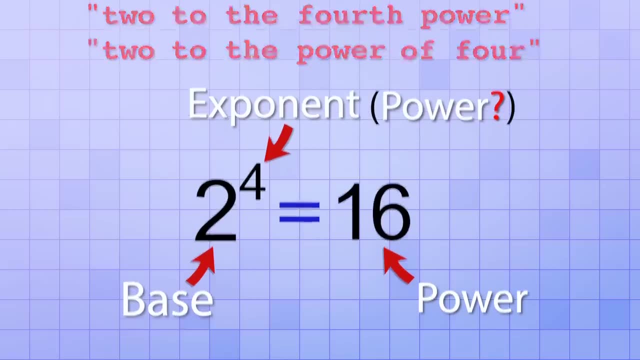 But when people started saying things like 2 to the 4th power or 2 to the power of 4,, it made it sound like the exponent was also called the power. The result is that nowadays you may hear people use the words exponent and power to mean the same thing. 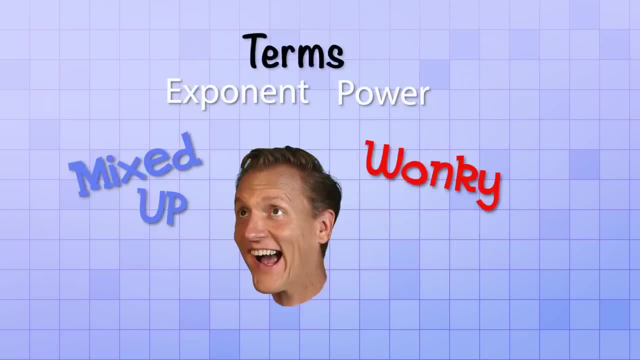 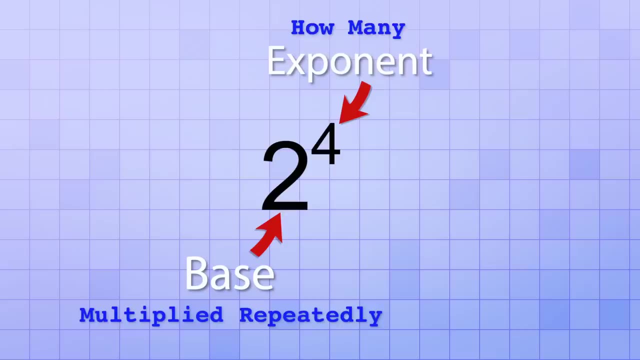 It's unfortunate that the terms have become so mixed up or wonky, but as long as you understand that the base is the number that gets multiplied repeatedly and the exponent tells you how many of them to multiply, you'll be in good shape. 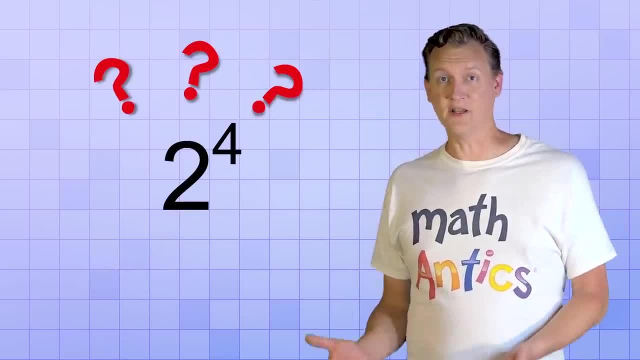 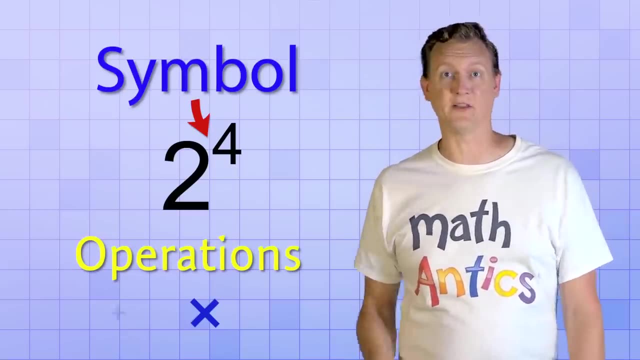 But I know what some of you are thinking…. Where is the operator symbol? If exponents are math operations, don't we need a symbol that goes between them, like there is with multiplication and the other arithmetic operations? Well, yes and no. 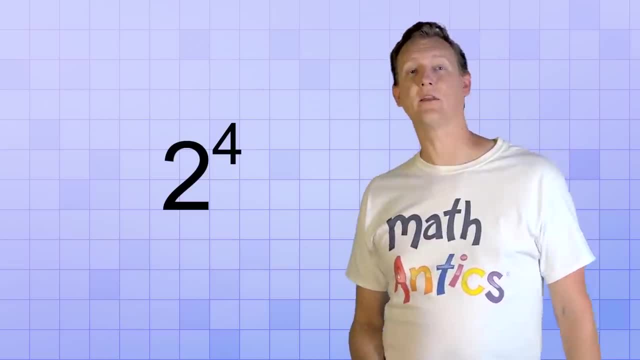 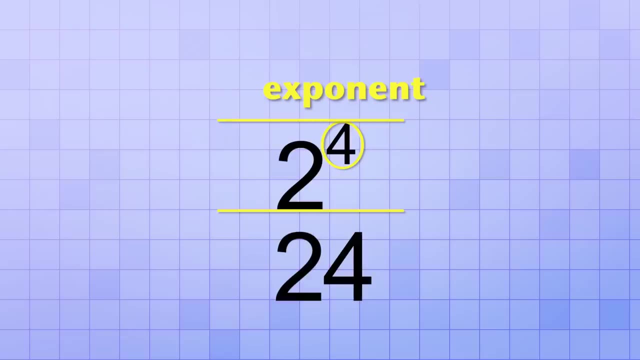 Most of the time we don't need a special operation symbol because of the way the numbers are written. Since the exponent is written smaller and up at the top of the line, it looks much different from a normal digit, so we don't need to use a symbol. 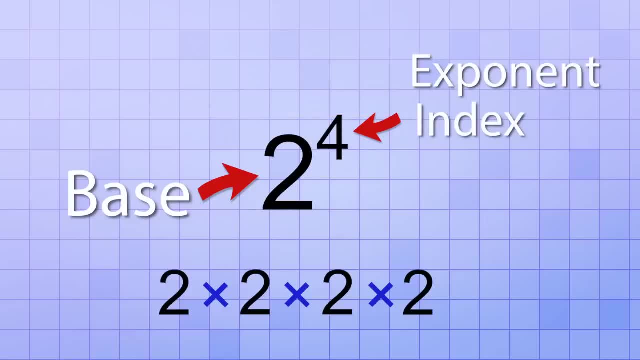 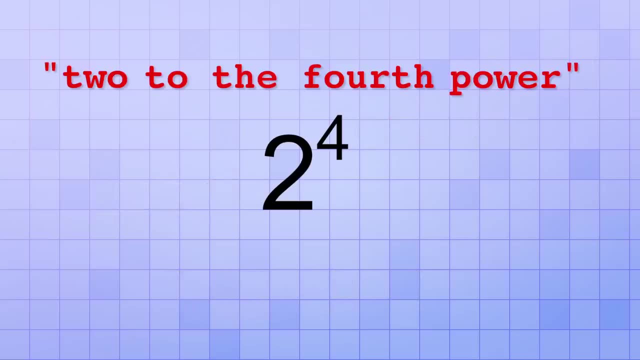 And it's called the exponent or the index, And when reading exponents some interesting terminology is used. This exponent would usually be read 2 to the 4th power, or just 2 to the 4th, for short. And this exponent would be read 3 to the 5th power, or just 3 to the 5th. 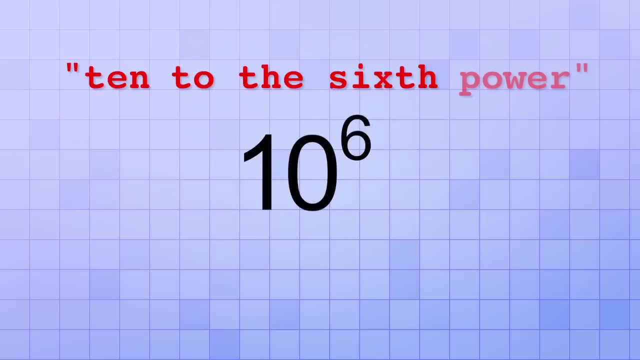 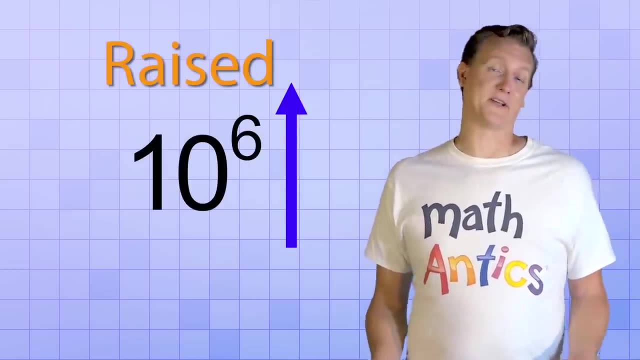 And this exponent would be read: 10 to the 6th power, or just 10 to the 6th, Get the idea? Oh, and you'll often hear people say that a number is raised to a certain power, You know cause. it sounds kinda cool. 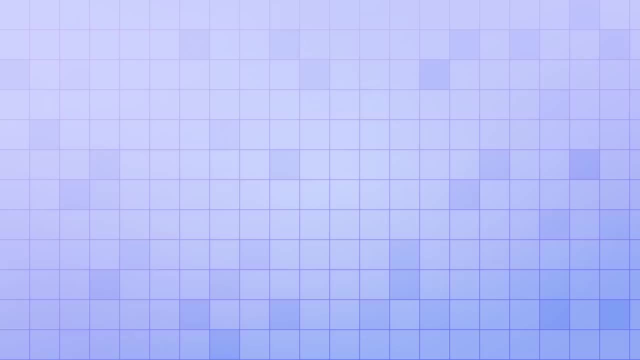 But it's just another way of saying the same thing. Unfortunately, that terminology has created a little confusion. Traditionally you'd say you have a base raised to a number, called an exponent, and the answer you get by doing that is called a power of that base. 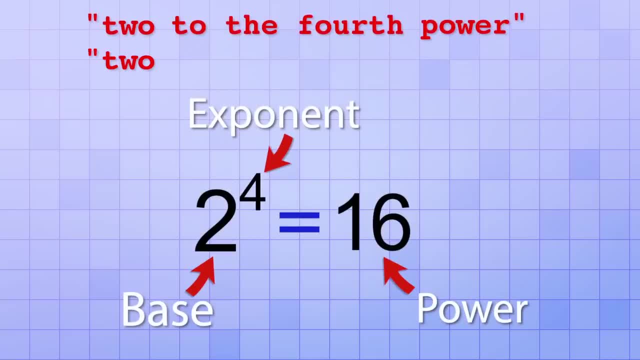 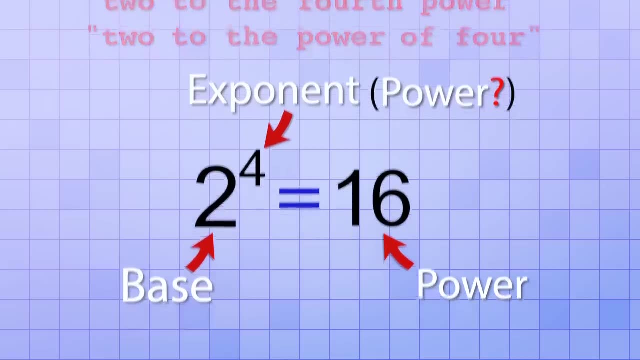 But when people started saying things like 2 to the 4th power or 2 to the power of 4,, it made it sound like the exponent was also called the power. The result is that nowadays you may hear people use the words exponent and power to mean the same thing. 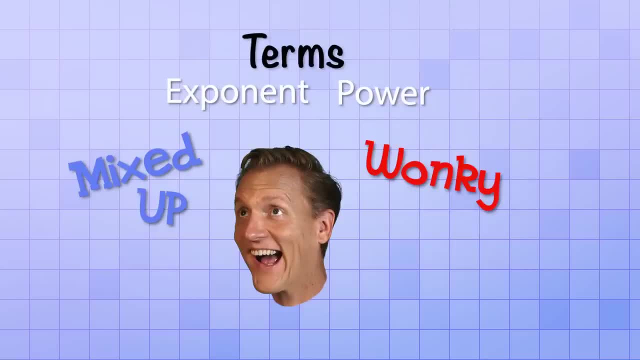 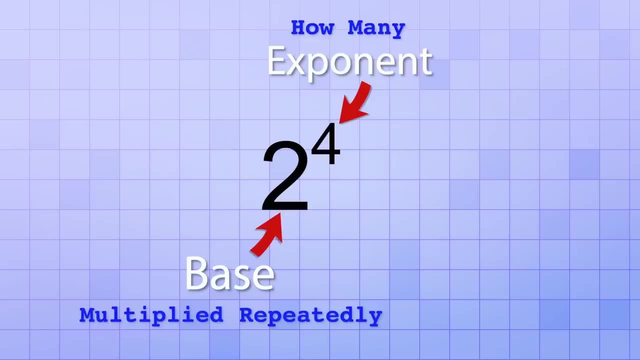 It's unfortunate that the terms have become so mixed up or wonky, but as long as you understand that the base is the number that gets multiplied repeatedly and the exponent tells you how many of them to multiply, you'll be in good shape. But I know what some of you are thinking. 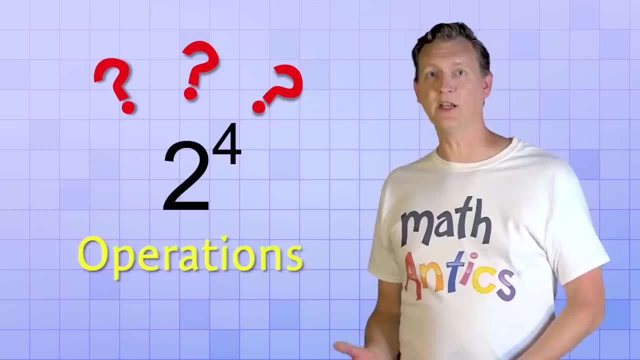 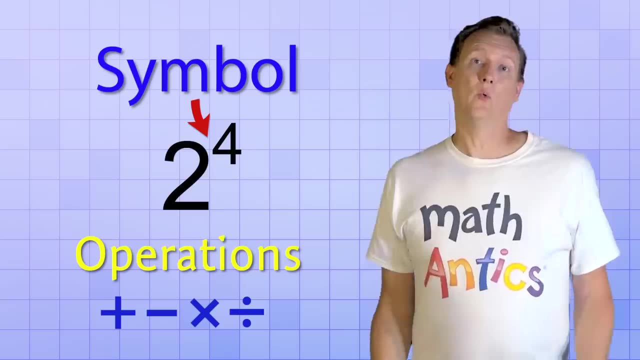 Where is the operator symbol? If exponents are math operations, don't we need a symbol that goes between them, Like there is with multiplication and the other arithmetic operations? Well, yes and no, Most of the time, we don't need a special operation symbol. 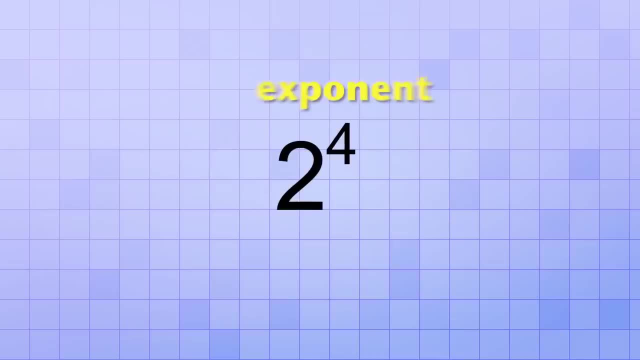 because of the way the numbers are written. Since the exponent is written smaller and up at the top of the line, it looks much different from a normal digit. so we don't need to use a symbol In math whenever you see a regular sized number with a smaller number up and to the right. 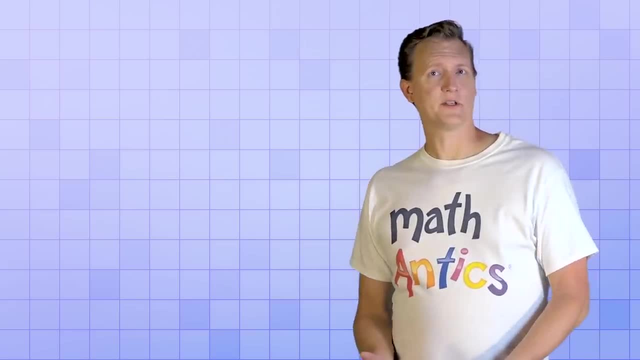 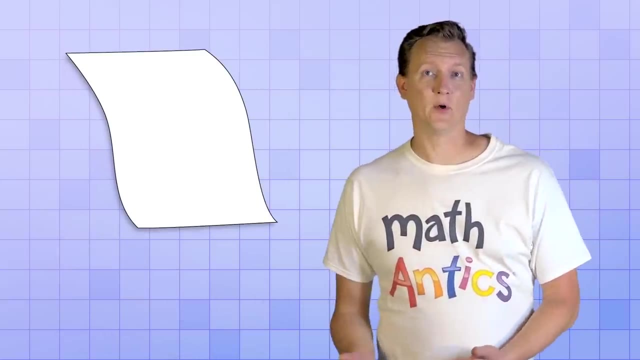 you know it's an exponent And once you get used to seeing exponents like this, it's easy to recognize them. The only real concern is when writing exponents down on paper, when you're trying to solve problems, If you're not careful or have really messy handwriting. 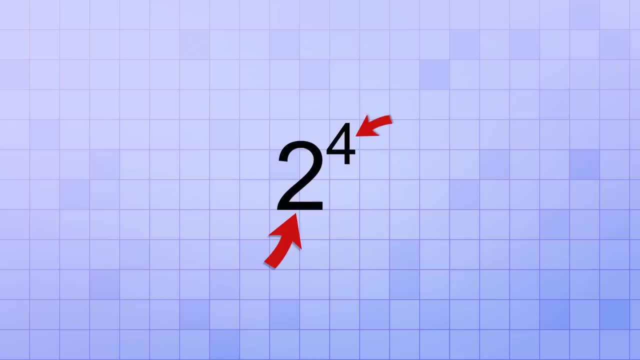 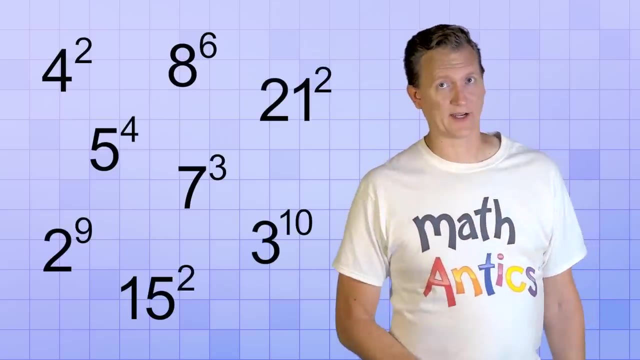 In math, whenever you see a regular sized number with a smaller number up and to the right, you know it's an exponent, And once you get used to seeing exponents like this, it's easy to recognize them. The only real concern is when writing exponents down on paper when you're trying to solve problems. 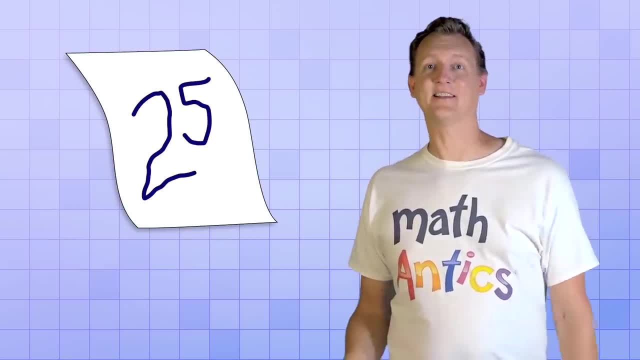 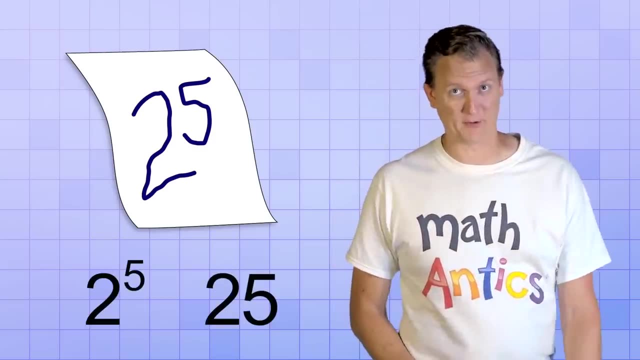 If you're not careful or have really messy handwriting, you might accidentally confuse an exponent like 2 to the 5th with a 2-digit number like 25. And obviously that would be a problem. But even if you're careful when writing exponents. 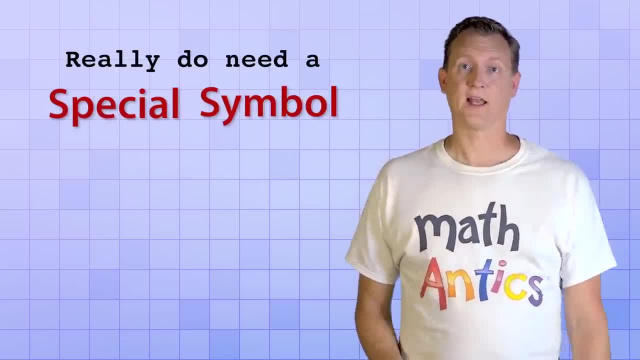 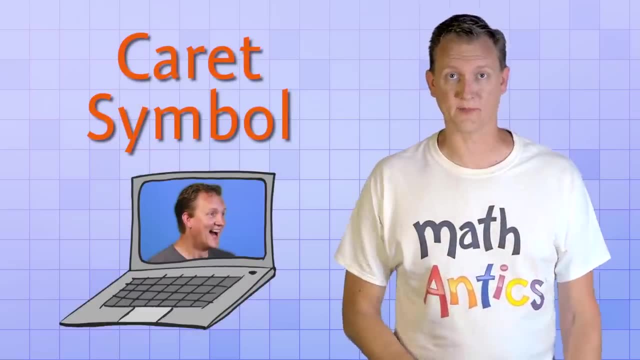 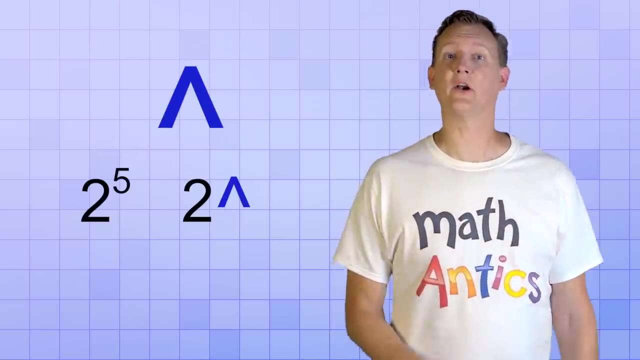 there are some times when you really do need a special symbol, Like when you type an exponent into a computer. In that case it's very common to use the caret symbol as the exponent operator. The caret symbol looks like this: So 2 to the 5th power would be written as 2 caret 5.. 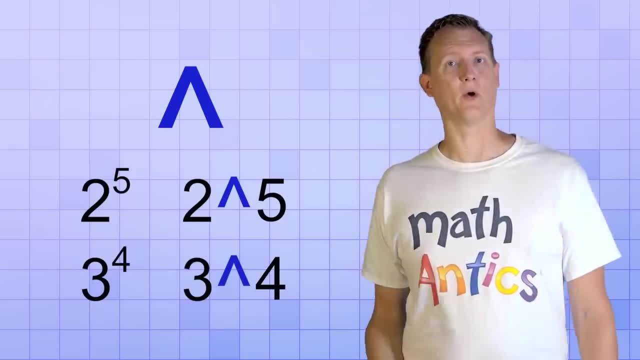 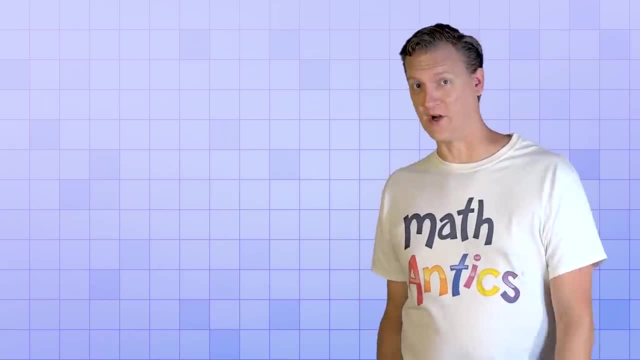 And 3 to the 4th power would be written as 3, caret, 4.. And that notation is used all the time in computer programming. Oh, and one more thing you should know before we move on is that exponent operations do NOT have the commutative property. 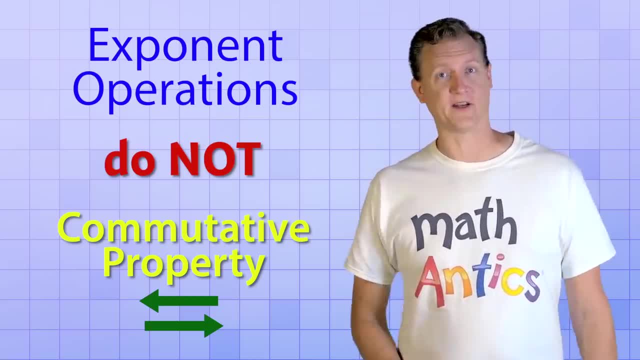 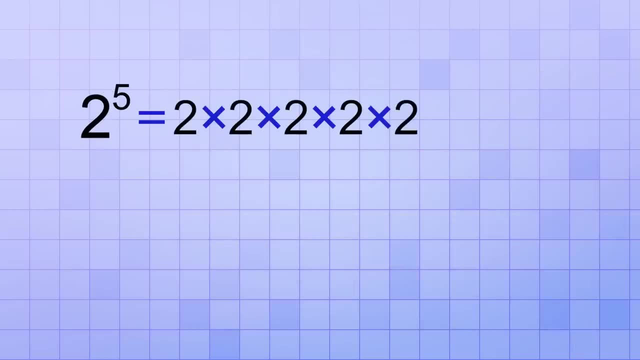 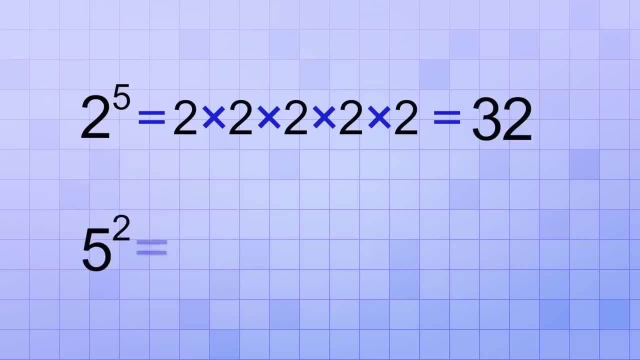 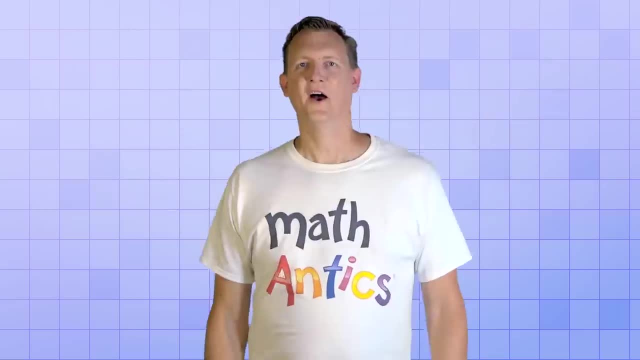 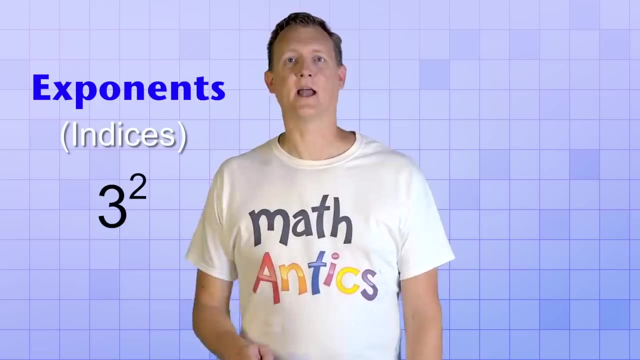 But if we switch the numbers 5 to the 2nd, power is 5 times 5, which equals 25.. So exponents do NOT have the commutative property. Okay, now that you know what exponents are and you know how they're written, it's time to talk about how they're used in math. 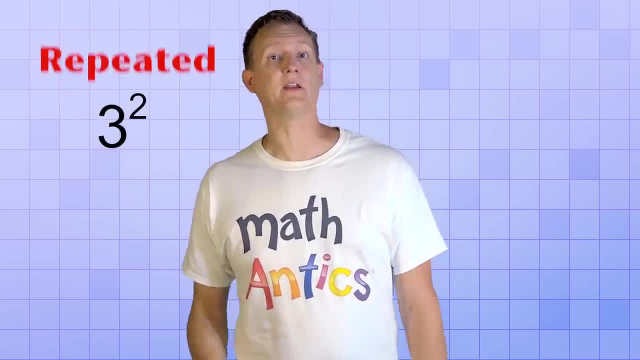 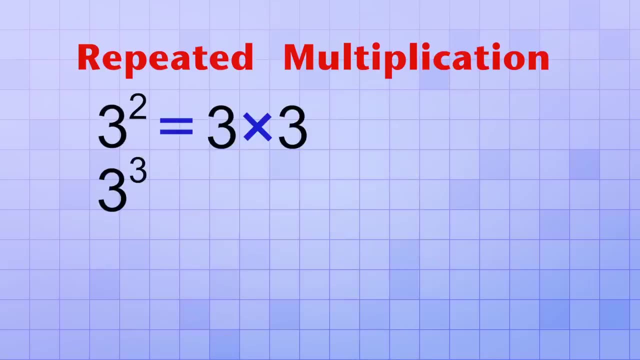 As I mentioned earlier, exponents are a way of doing repeated multiplication. 3 to the 2nd power is the same as 3 times 3.. 3 to the 3rd power is the same as 3 times 3.. 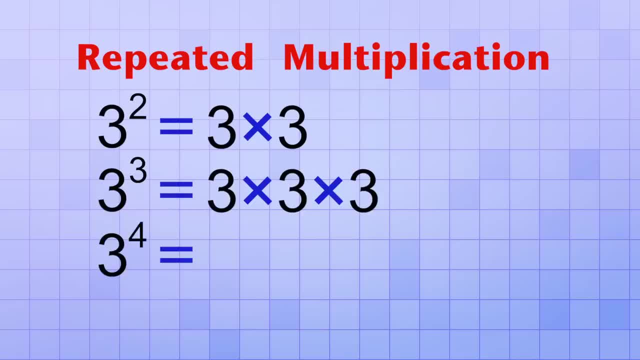 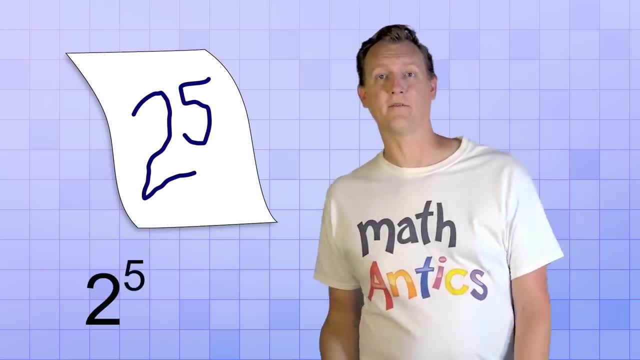 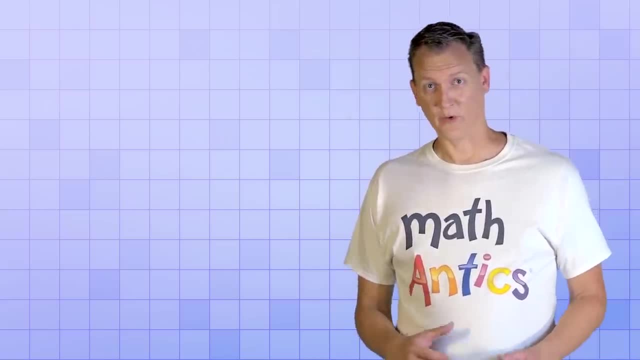 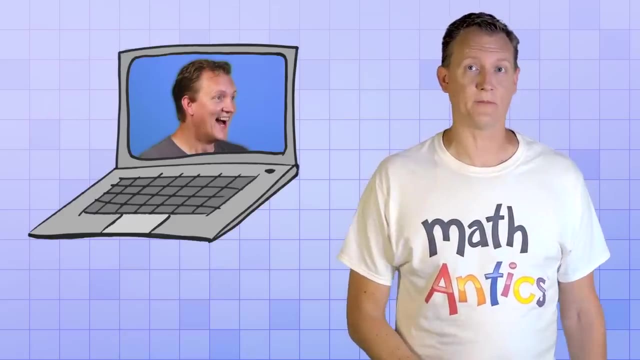 you might accidentally confuse an exponent with a two-digit number And obviously that would be a problem. But even if you're careful when writing exponents, there are some times when you really do need a special symbol, Like when you type an exponent into a computer. 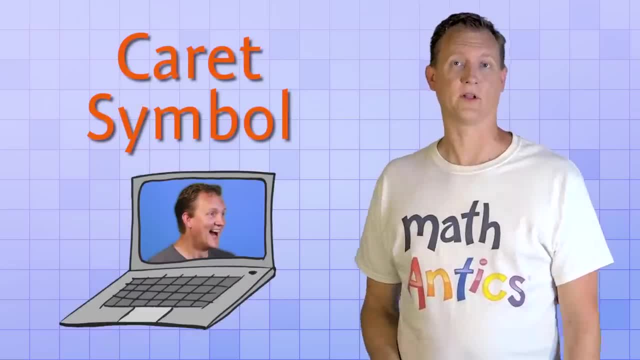 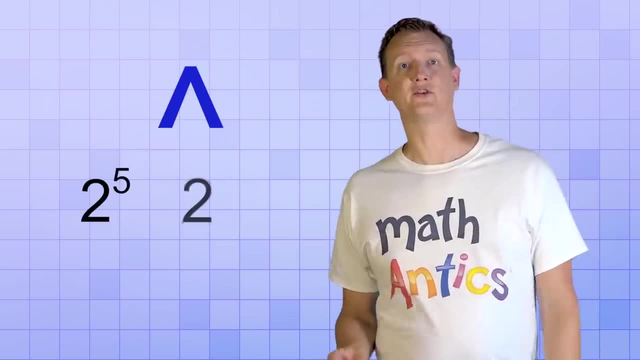 In that case it's very common to use the caret symbol as the exponent operator. The caret symbol looks like this: So 2 to the 5th power would be written as 2 caret 5.. And 3 to the 4th power would be written as 3 caret 4.. 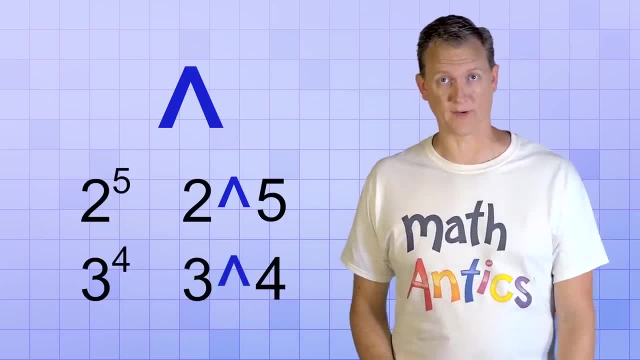 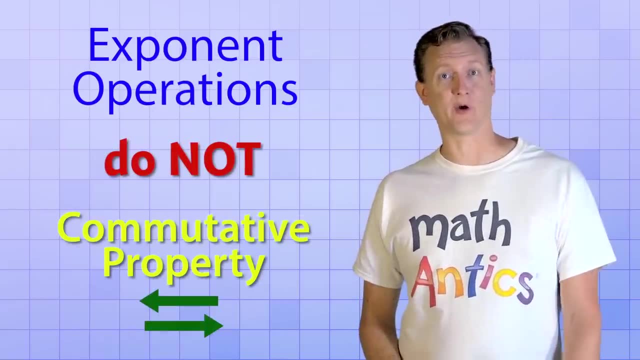 And that notation is used all the time in computer programming. Oh, and one more thing you should know before we move on is that exponent operations do NOT have the commutative property. In other words, you can't switch the order of the numbers without getting a different answer. 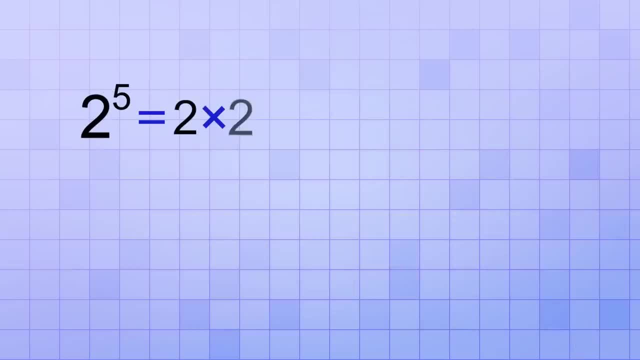 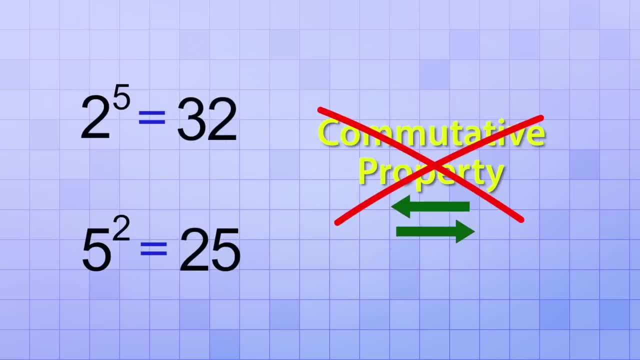 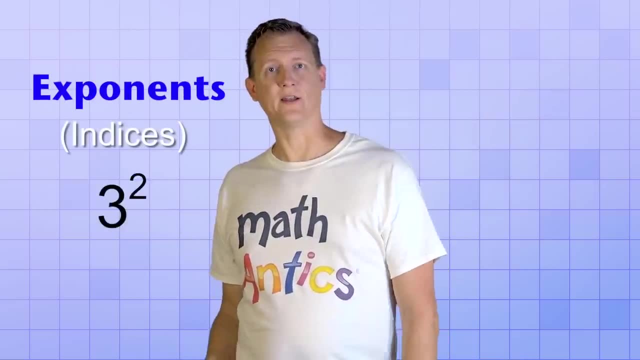 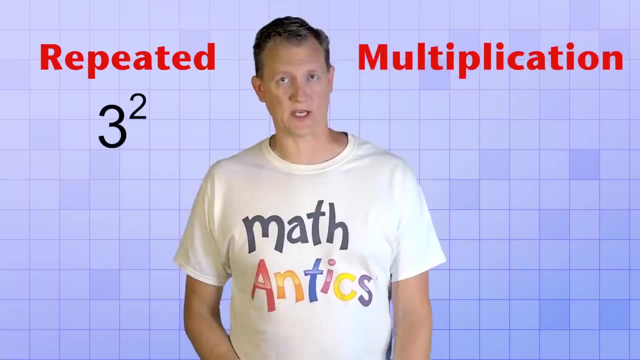 So exponents do NOT have the commutative property. Okay, now that you know what exponents are- or indices if you prefer- and you know how they're written, it's time to talk about how they're used in math. As I mentioned earlier, exponents are a way of doing repeated multiplication. 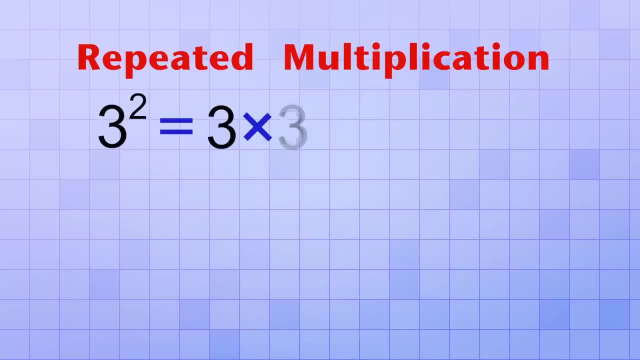 3 to the 2nd power is the same as 3 times 3.. 3 to the 3rd power is the same as 3 times 3 times 3.. 3 to the 4th power is the same as 3 times 3 times 3 times 3.. 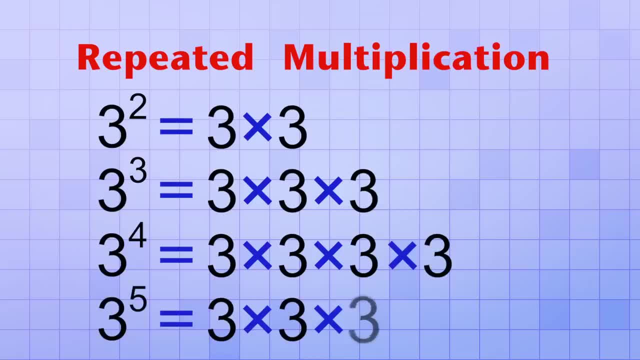 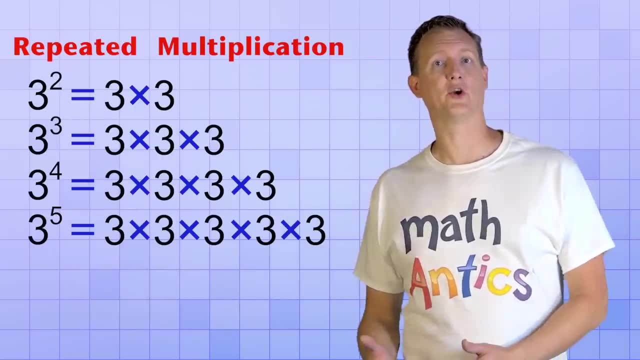 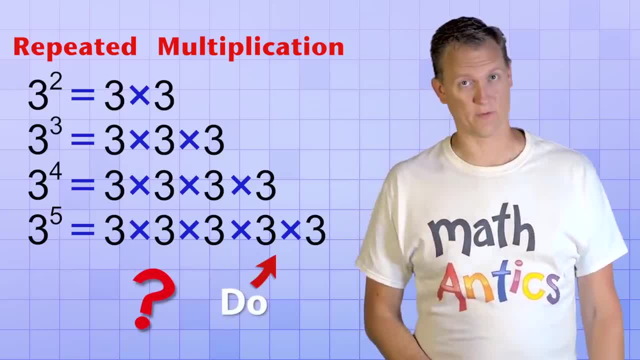 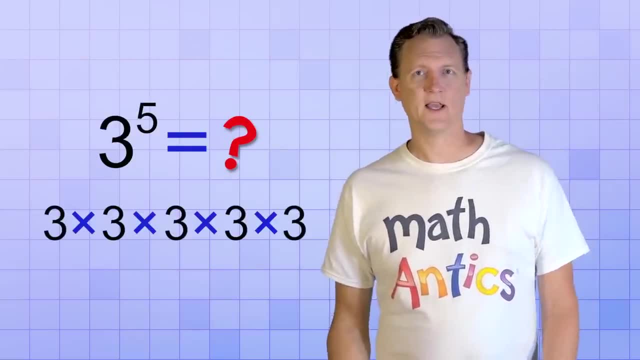 Do exponents help then? Well, yes and no. If you have to actually figure out what 3 to the 5th power is, you still need to multiply 3 together 5 times, and you could do that by hand, or you could use a calculator to help you. 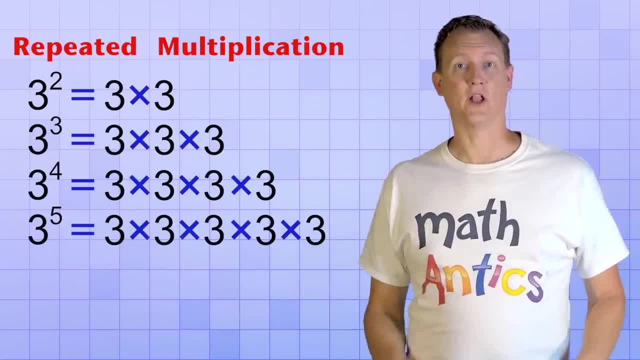 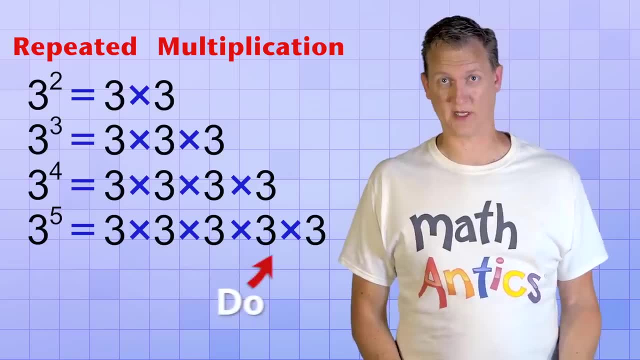 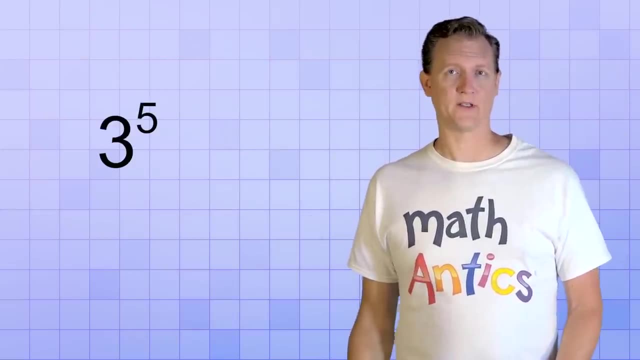 See the pattern. So exponents can save you a lot of writing when you need to show repeated multiplication, But what about when you actually need to DO repeated multiplication? Do exponents help then? Well, yes and no, If you have to actually figure out what 3 to the 5th power is. 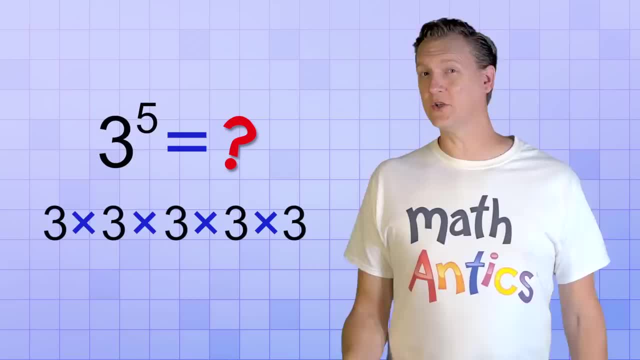 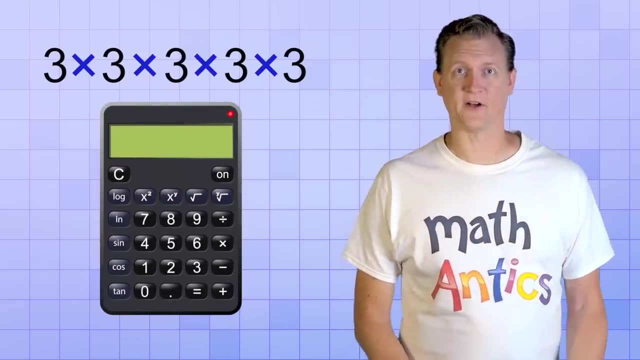 you still need to multiply 3 together 5 times, and you could do that by hand or you could use a calculator to help you. In fact, if you have a multi-function or scientific calculator, it might have a button on it that looks something like this: 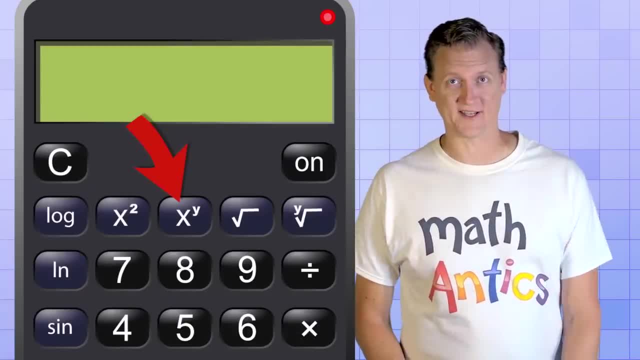 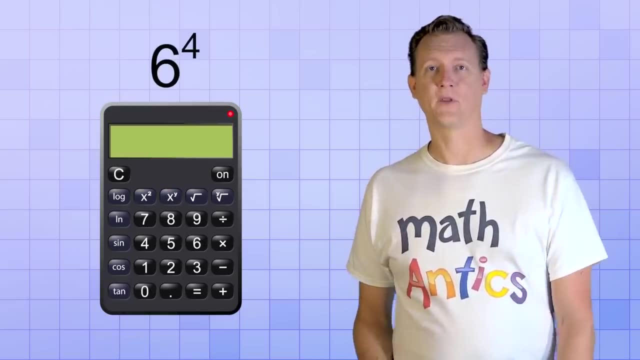 X to the power of Y, which makes calculating exponents really easy. Let's try using that calculator function to figure out what this exponent would be: 6 to the 4th power, which is the same as 4 sixes multiplied together. 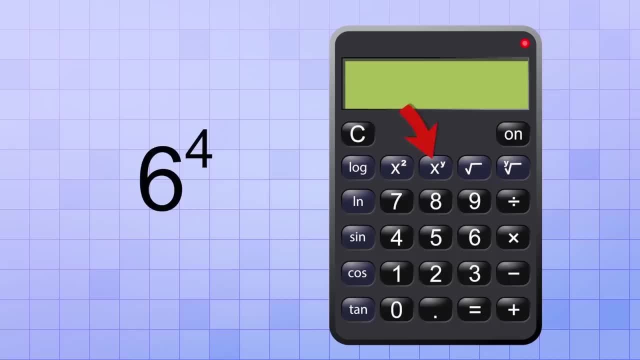 On most calculators. this is how the exponent button works. First you type in the number that's the base of your exponent. So in this problem we type in 6. And then you'd hit the exponent button, which might not do anything besides let the calculator know. 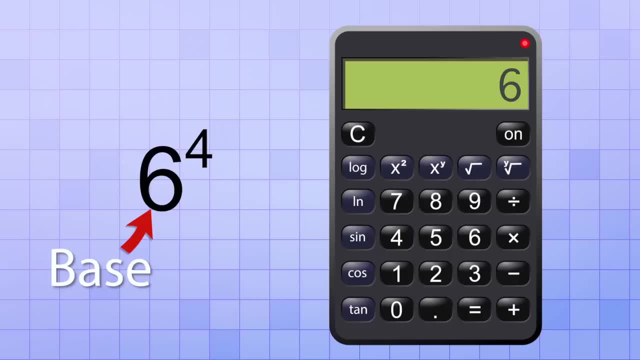 that the next number you give it will be an exponent. So next you enter the exponent, which is 4 in this case. Now all you have to do is hit the equal sign to get the answer, which is 1296.. Wow, As you can see, knowing how to do that with a calculator saved us a lot of work. 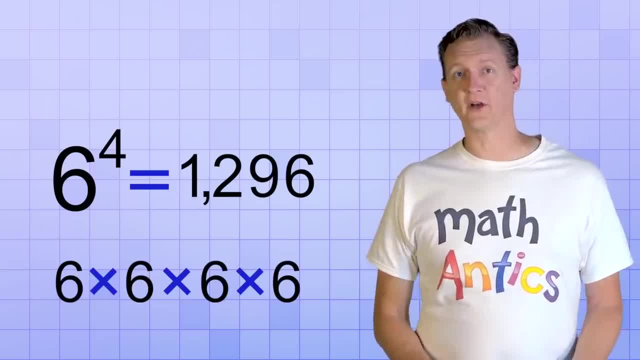 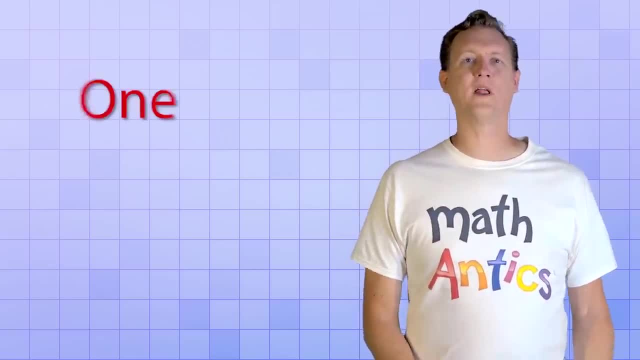 And now we know that 4 sixes multiplied together will be 1296.. In the examples we've seen so far, we've only had simple one-digit exponents like 2, 3 or 4.. But exponents can be any number. 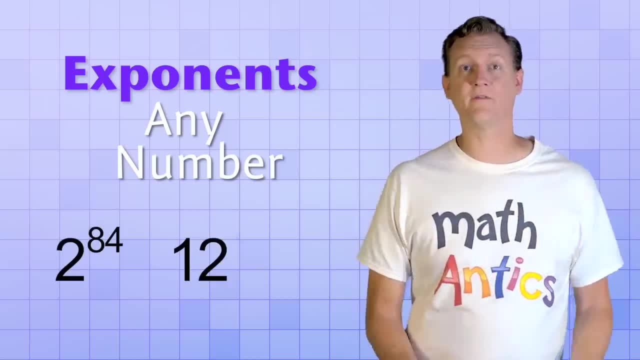 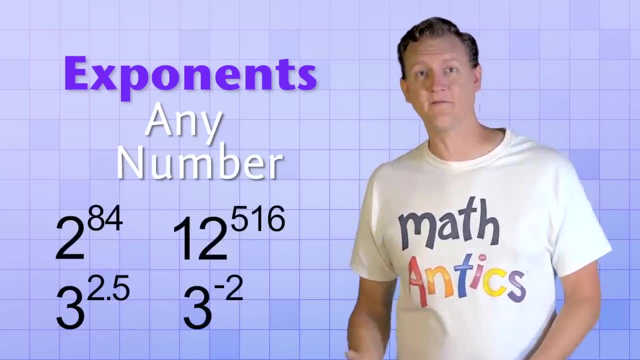 You could have 2 to the 84th power or 12 to the 516th power. In fact, as crazy as it sounds, you can even have exponents that are decimals or negative numbers, But we'll save advanced exponents like that for future videos. 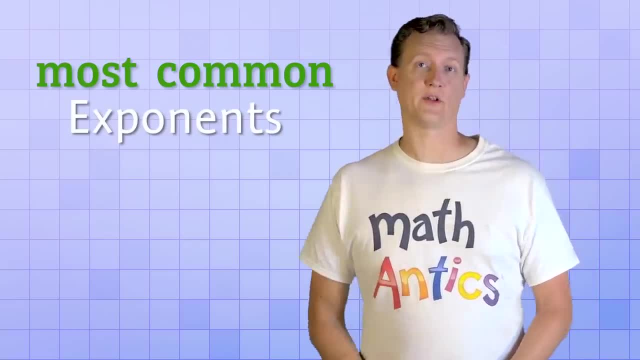 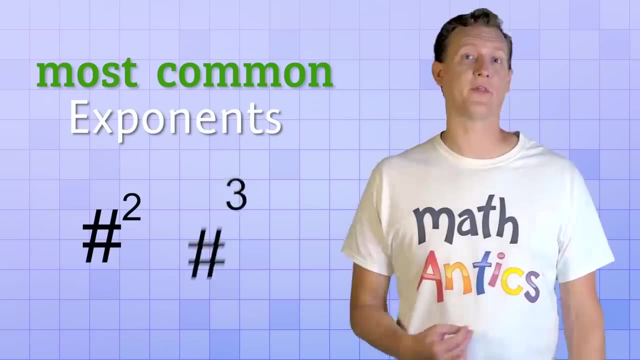 In the last part of this video, I want to focus on the two most common exponents you'll encounter, which are 2 and 3.. That is, you'll very often see a number raised to the 2nd power or to the 3rd power. 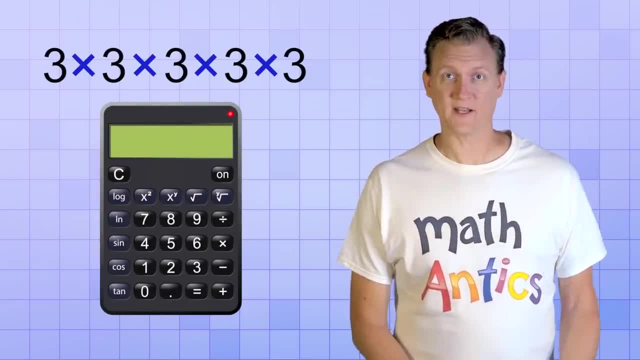 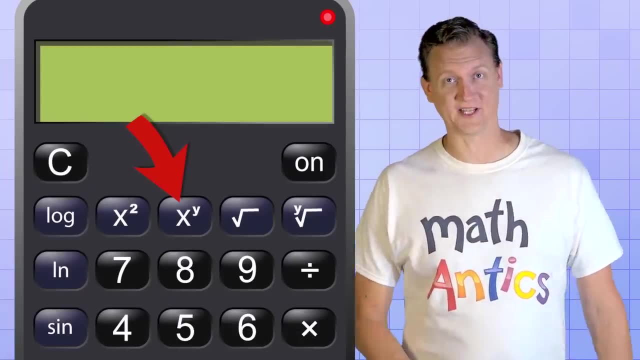 In fact, if you have a multifunction or scientific calculator, it might have a button on it that looks something like this: X to the power of Y, which makes calculating exponents really easy. Let's try using that calculator function to figure out what this exponent would be. 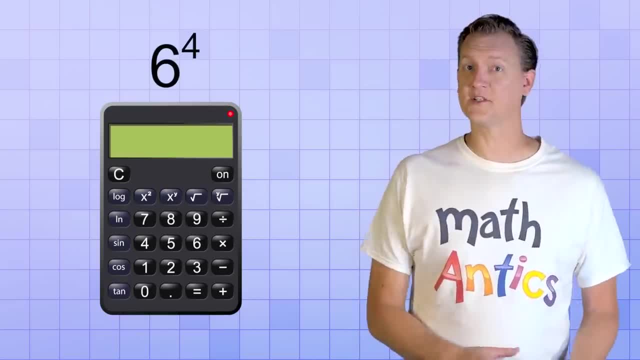 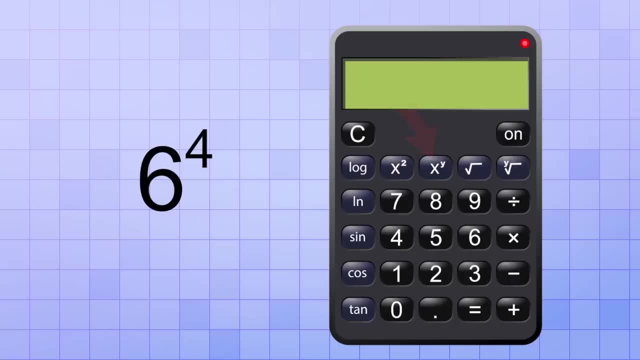 6 to the 4th, power, which is the same as 4 sixes multiplied together On most calculators. this is how the exponent button works. First you type in the number that's the base of your exponent. So in this problem we type in 6.. 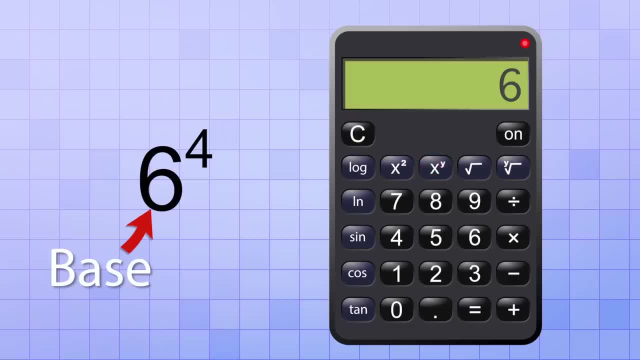 And then you'd hit the exponent button, which might not do anything besides let the calculator know that the next number you give it will be an exponent. So next you enter the exponent, which is 4 in this case. Now all you have to do is hit the equal sign to get the answer, which is 1296.. 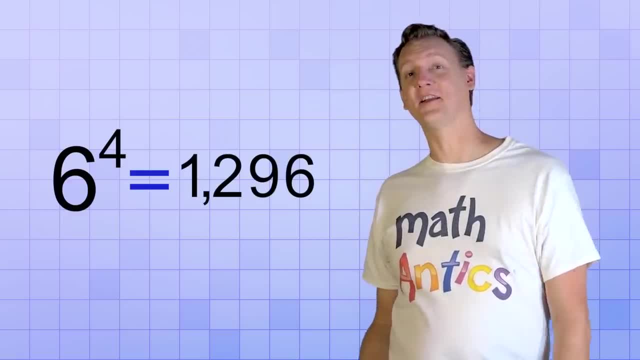 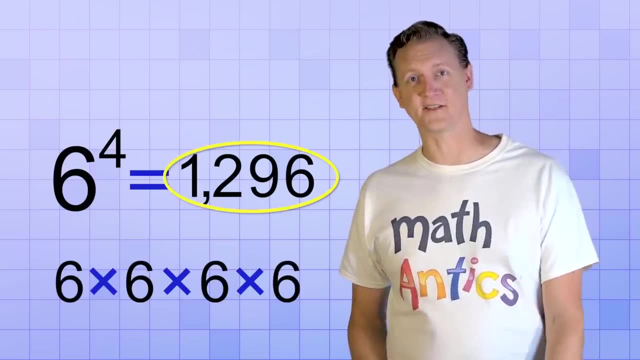 Wow. As you can see, knowing how to do that with a calculator saved us a lot of work, And now we know that 4 sixes multiplied together will be 1296.. In the examples we've seen so far, we've only had simple one-digit exponents. 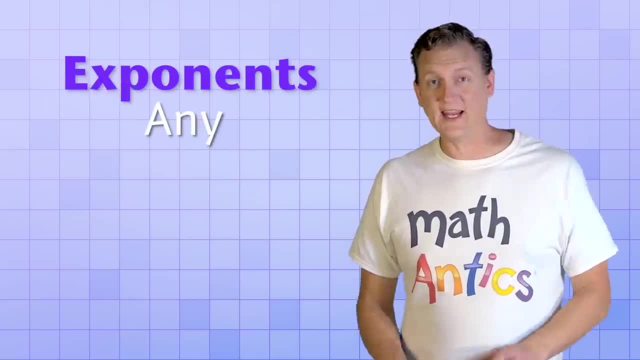 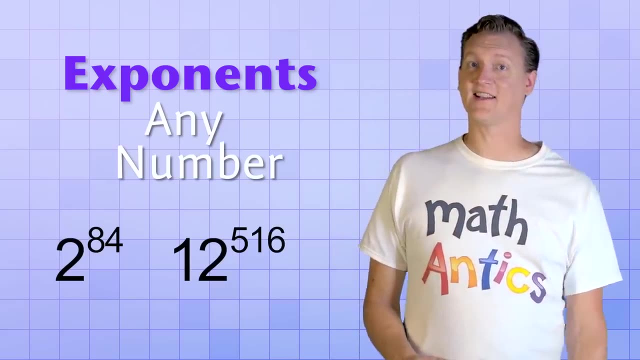 like 2, 3 or 4.. But exponents can be any number. You could have 2 to the 84th power or 12 to the 516th power. In fact, as crazy as it sounds, you can even have exponents that are decimals. 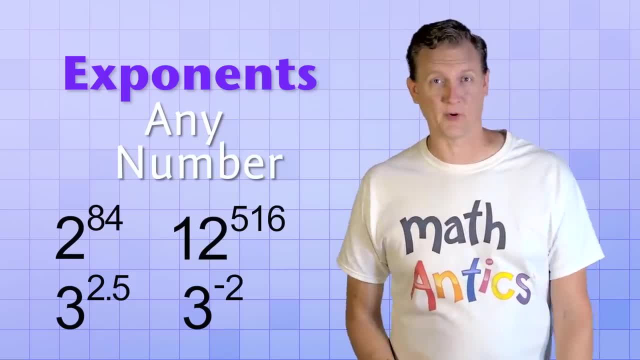 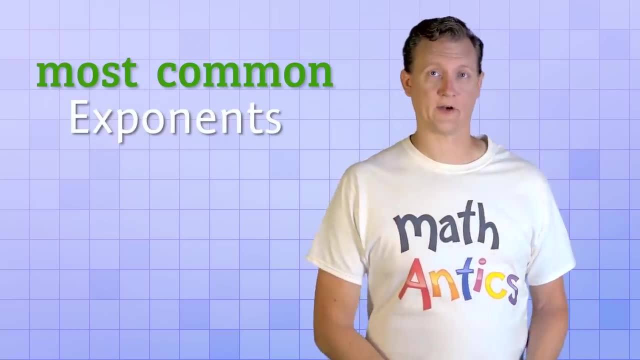 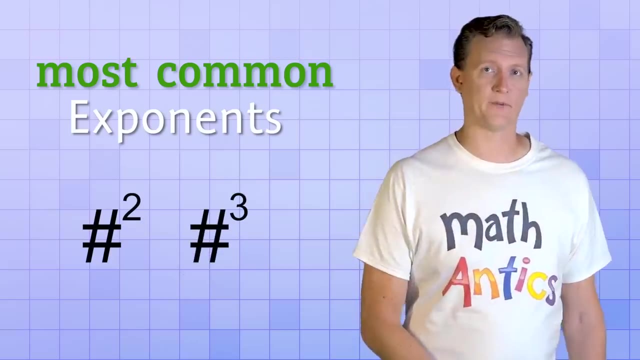 or negative numbers, But we'll save advanced exponents like that for future videos. In the last part of this video I want to focus on the two most common exponents you'll encounter, which are 2 and 3.. That is, you'll very often see a number raised to the 2nd power or to the 3rd power. 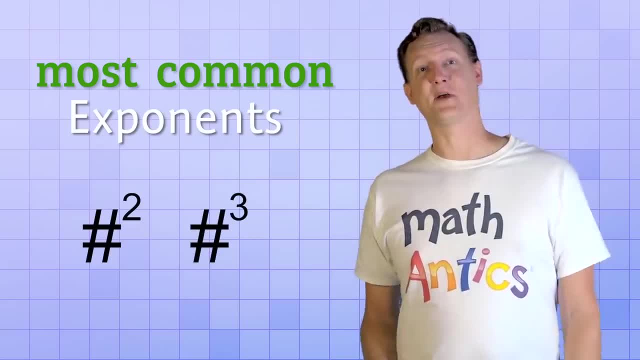 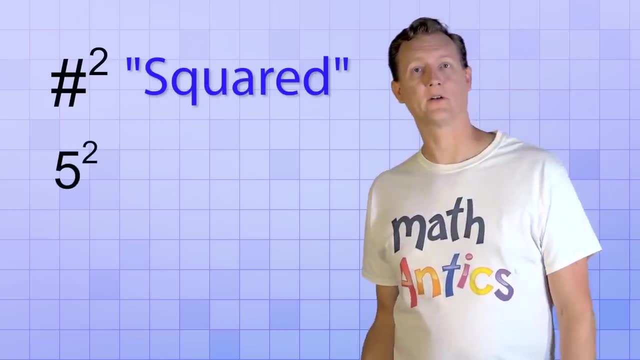 In fact, those exponents are so common that they even have special names. When a number is raised to the 2nd power, we say it's being squared. So 5 to the 2nd power is also referred to as 5 squared. 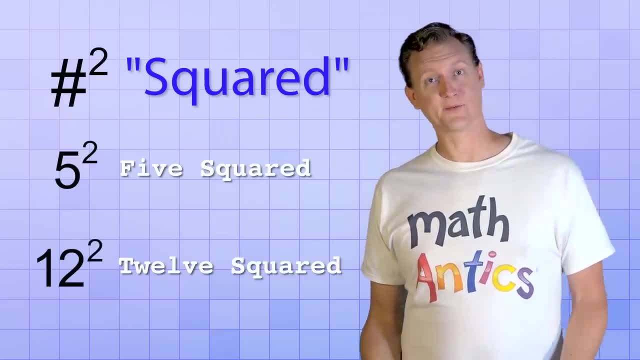 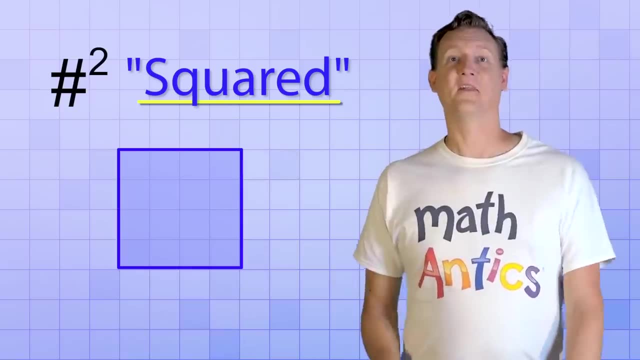 And 12 to the 2nd power would be 12 squared. Now, if you're new to exponents, that might sound kind of funny, But can you think of a reason why the term squared is used? Yep, that's how you'd calculate the area of a square shape. 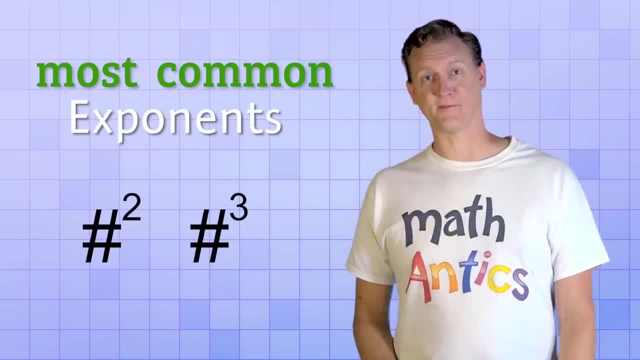 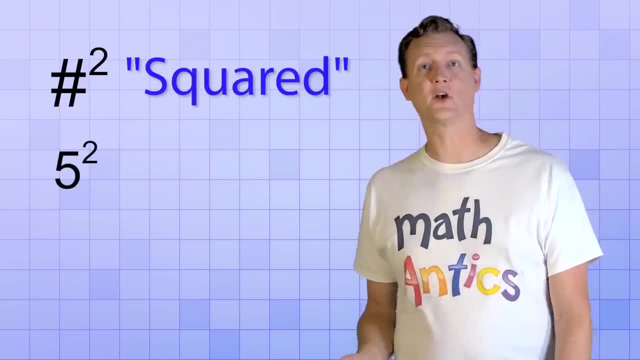 In fact, those exponents are so common that they even have special names. When a number is raised to the 2nd power, we say it's being squared. So 5 to the 2nd power is also referred to as 5 squared. 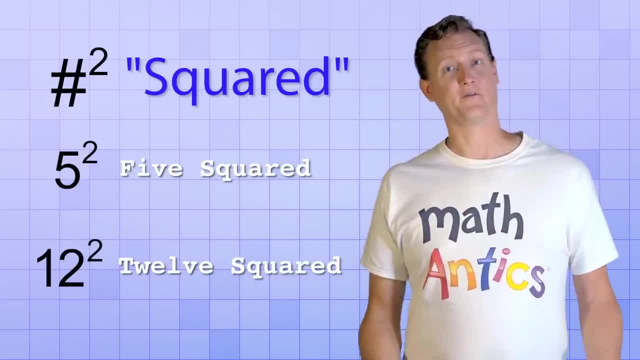 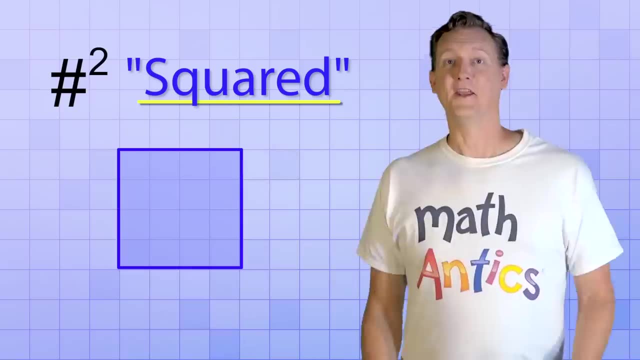 And 12 to the 2nd power would be 12 squared. Now, if you're new to exponents, that might sound kind of funny, But can you think of a reason why the term squared is used? Yep, that's how you'd calculate the area of a square shape. 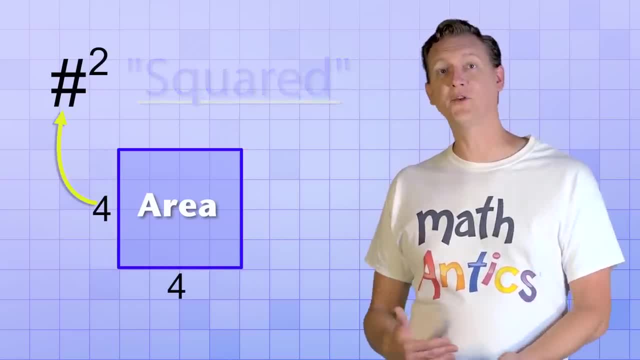 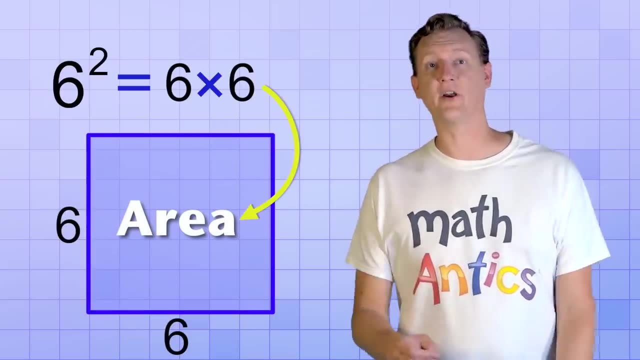 Since squares have sides that are all the same length, if you multiply that length together twice, like 4 times 4 or 5 times 5 or 6 times 6, it gives you the area of that square. And it's a similar story for numbers that are raised to the 3rd power. 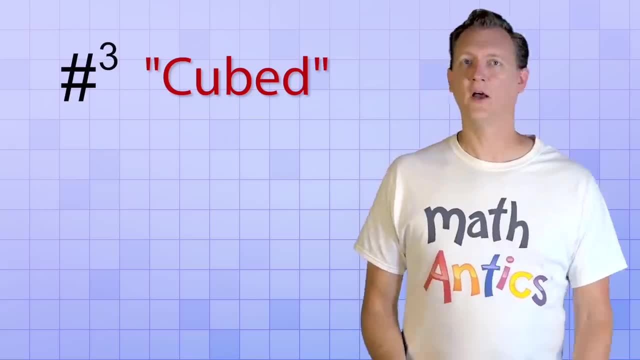 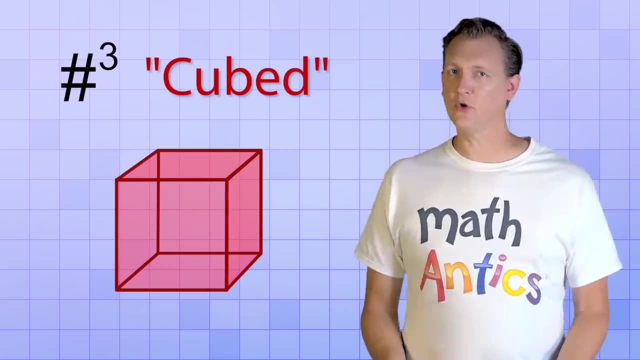 In that case you'd say that the number is being cubed. So 5 to the 3rd power is also 5 cubed, And 8 to the 3rd power would be 8 cubed, Since cubes are 3-dimensional objects with sides that are all the same length. 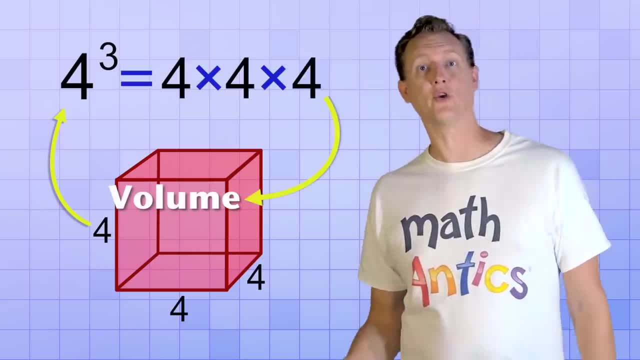 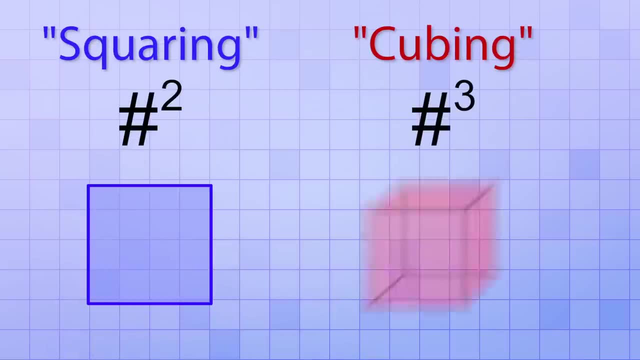 if you multiply that length together 3 times you would get the volume of the cube. So squaring a number gets its name from squares And cubing a number gets its name from cubes. And that helps explain why the exponents 2 and 3. 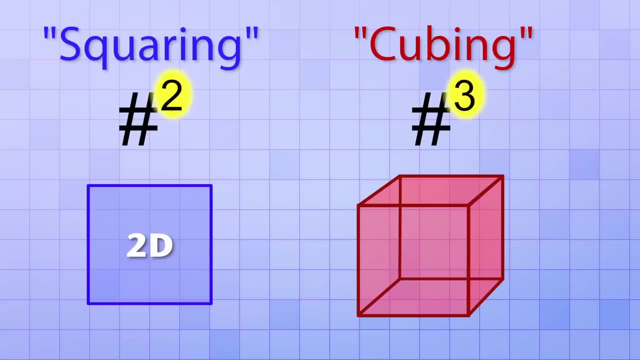 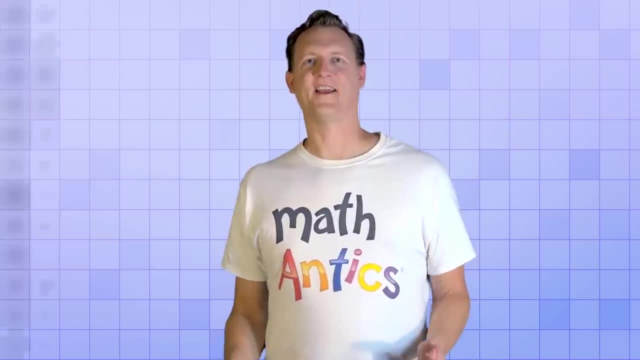 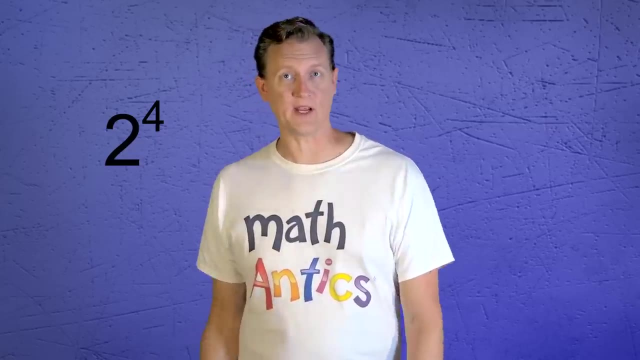 are really common in math. Because we interact with 2- and 3-dimensional objects all the time in the real world, there are lots of practical applications. Okay, so now you know that exponents are a way of showing repeated multiplication, and you also know what the two numbers in an exponent mean. 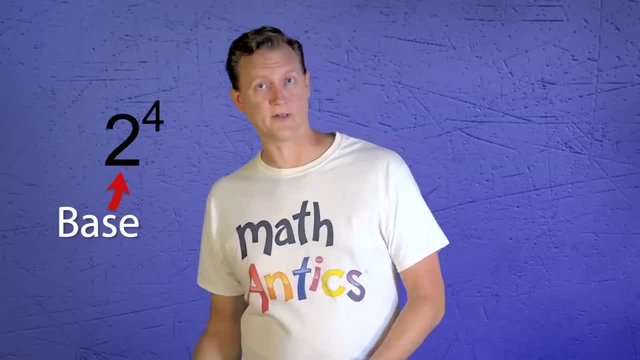 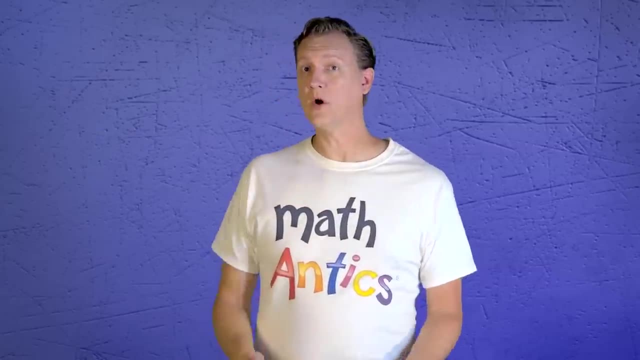 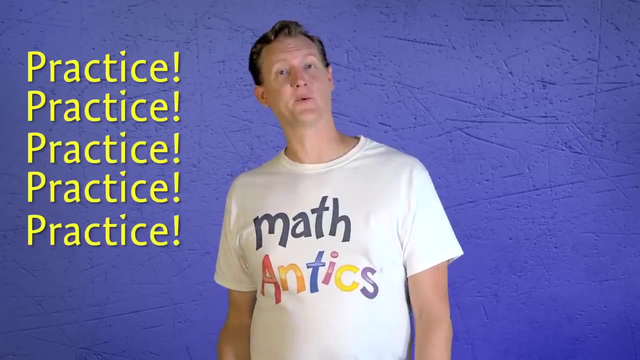 The base is the number that will get repeatedly multiplied together and the exponent tells us how many times to repeat it. In the next video, we'll learn more about exponents and their inverse operations, called roots. Learning math takes a lot of practice, so be sure to practice what you've learned in this video. Thanks for watching Math Antics and I'll see you next time.